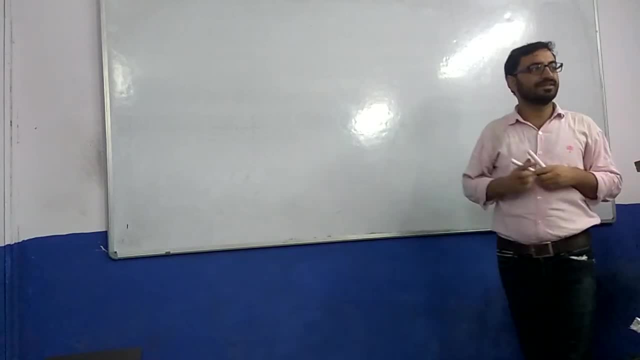 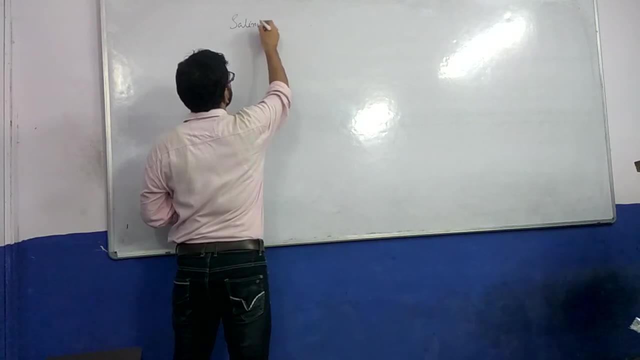 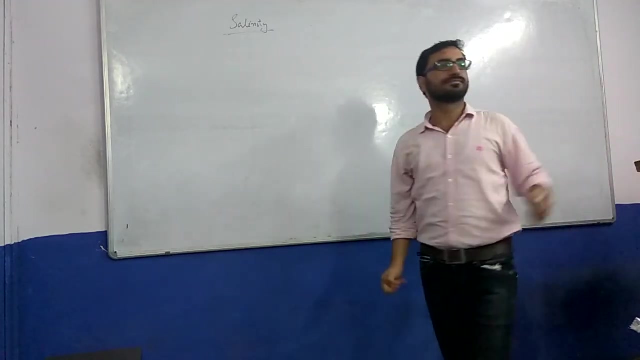 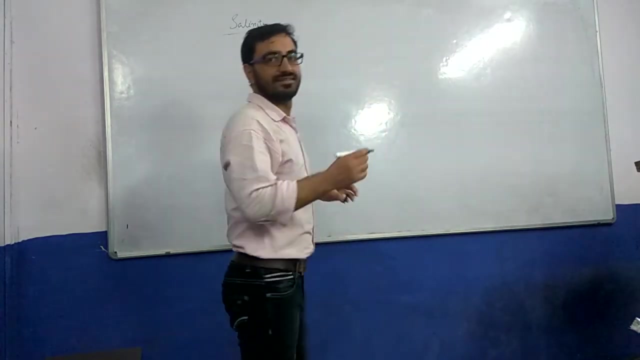 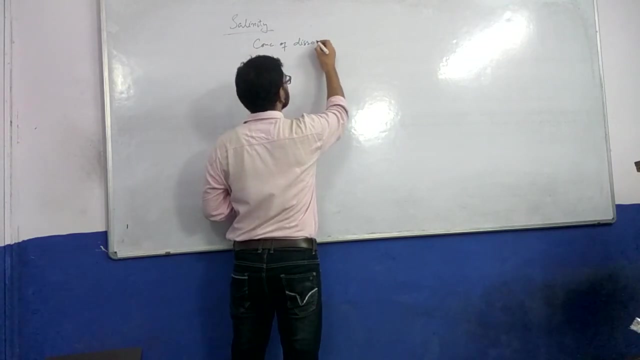 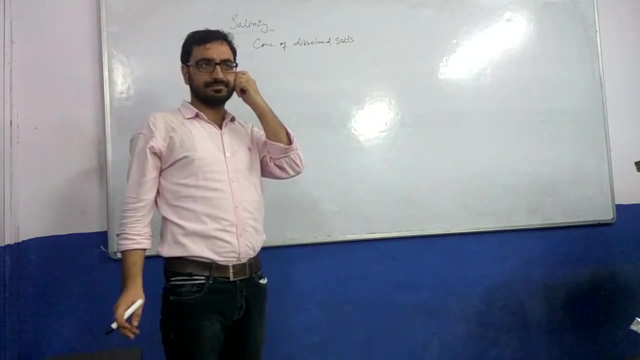 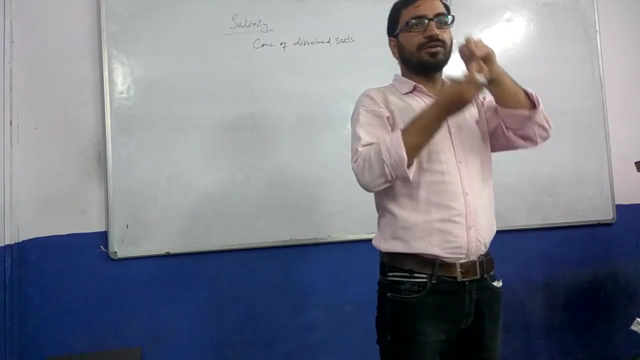 Okay, now let us see salinity. What is salinity? Hey, don't talk. What is salinity? It is the concentration of dissolved salts. It is the concentration of dissolved salts. It is the ratio of the weight of the salts to the weight of the water. 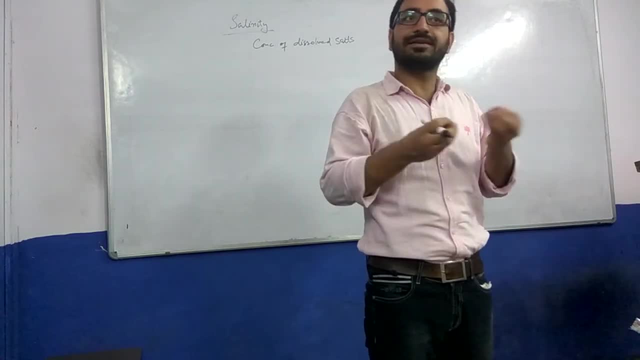 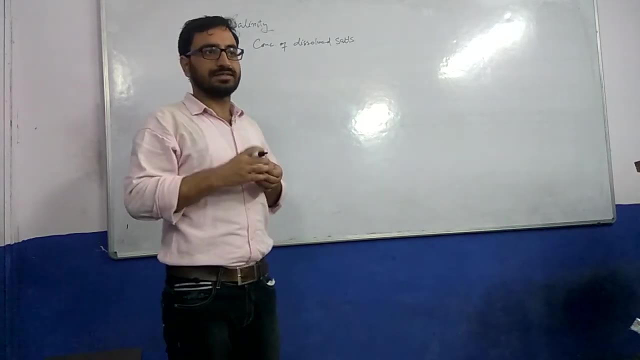 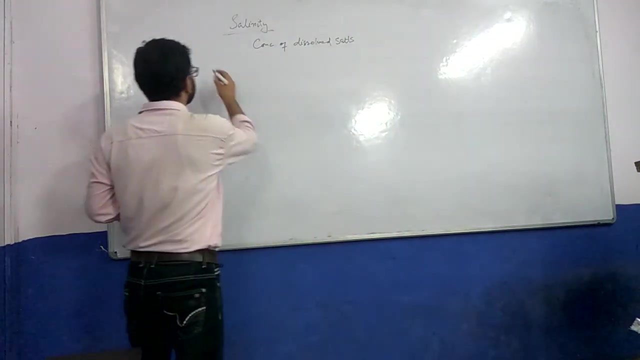 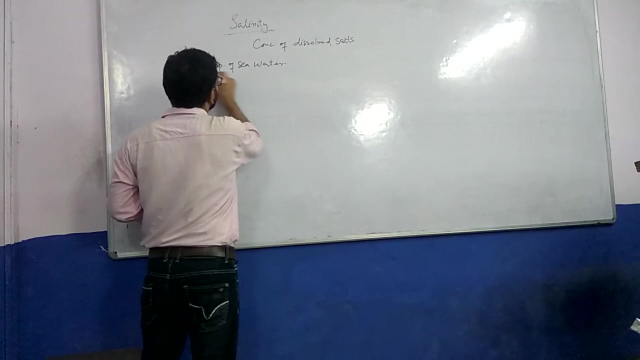 How much salt is in how much water. That is the salinity, Because water is the solvent, It is an active solvent. Seawater is the active solvent. So, before going there, let us see the composition of seawater. Let us see the composition of seawater. What is the composition of seawater? 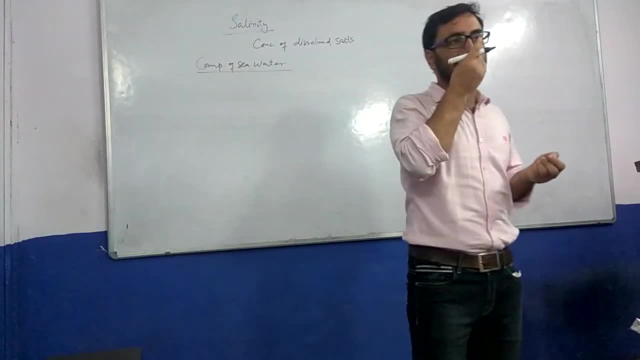 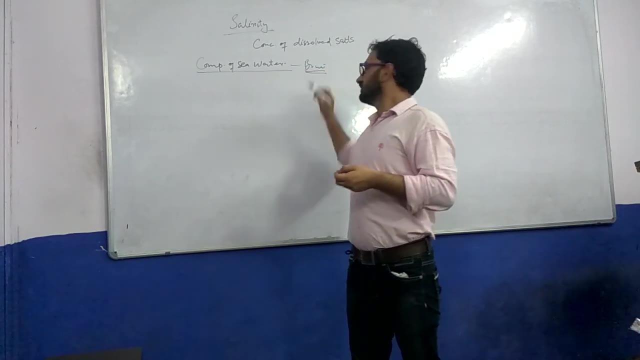 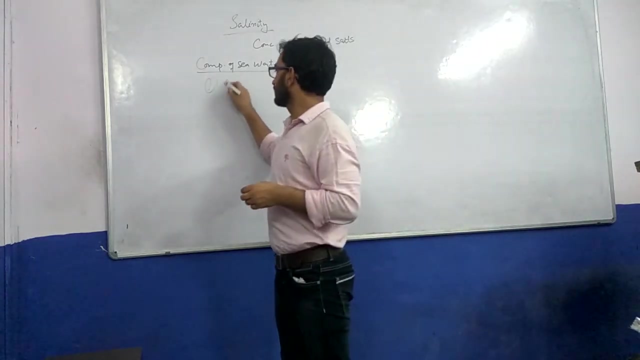 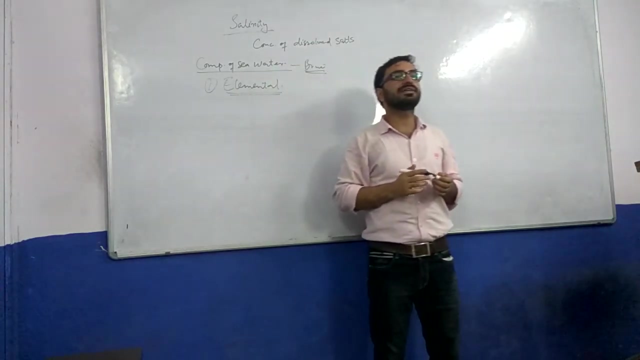 Seawater is a mixture of so many things. so many salts are there. It is a brine. We call it a brine, So first of all, write the elemental composition. Elemental composition: Which element is more in seawater and which is less? 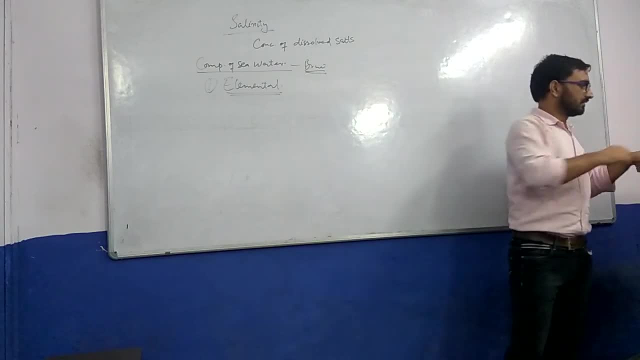 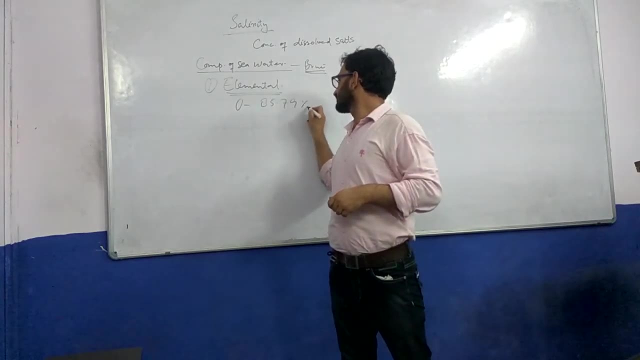 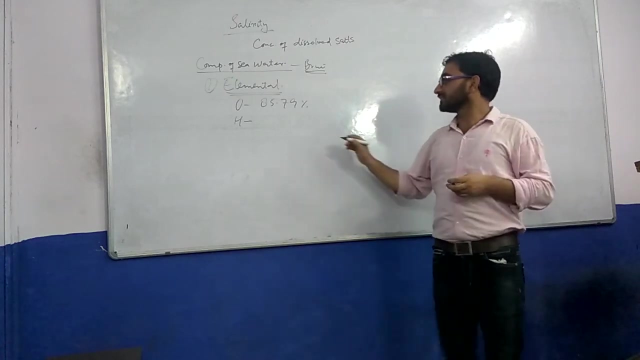 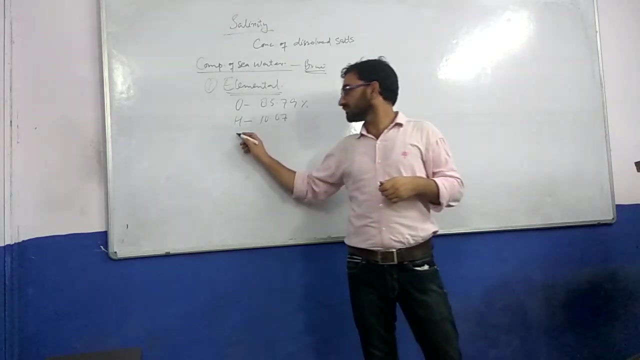 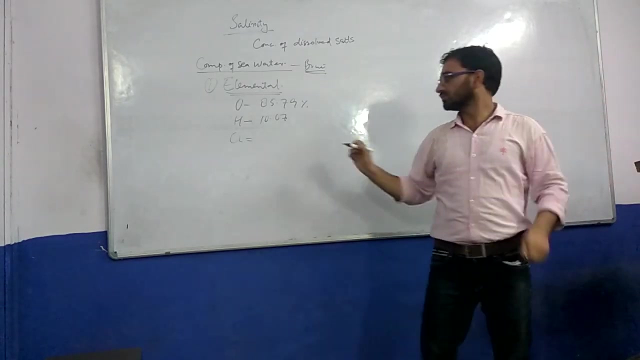 First of all write oxygen: 85.79%- 85.79%. After that look at hydrogen 10.67%. After hydrogen you write it is chlorine. It is chlorine 1.92.. Then it is sodium. 1.07%, Then it is magnesium 0.13%. Magnesium 0.13%. Magnesium 0.13%. Then it is sulphur. Then it is sulphur 0.08%, Then it is sulphur. 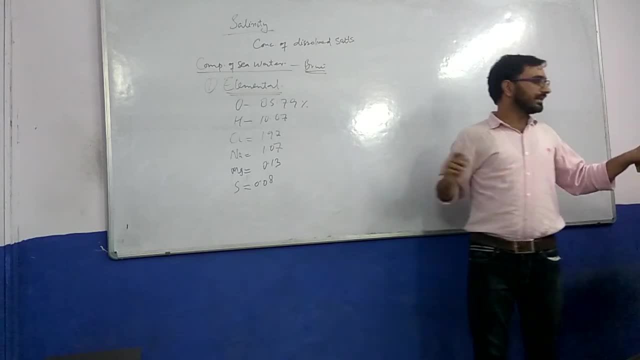 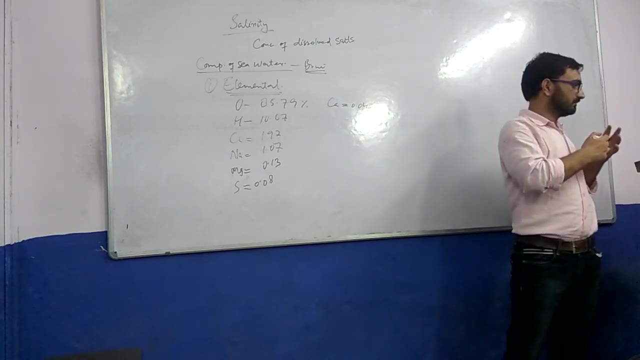 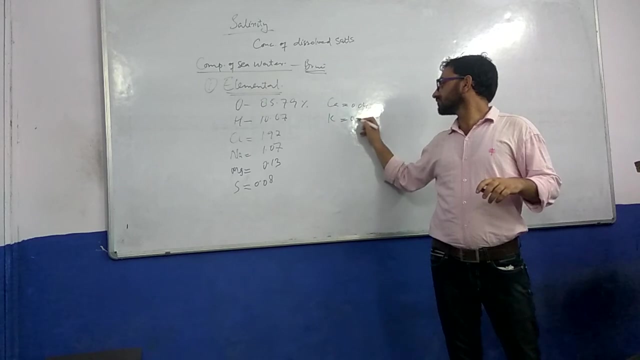 0.08%. After sulphur, write calcium: 0.04%, 0.04%, 0.04%, Then write potassium: 0.03%, Then write potassium: 0.03%, 0.03%, 0.03%. 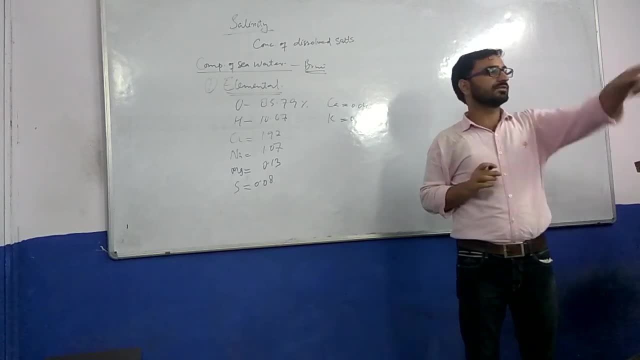 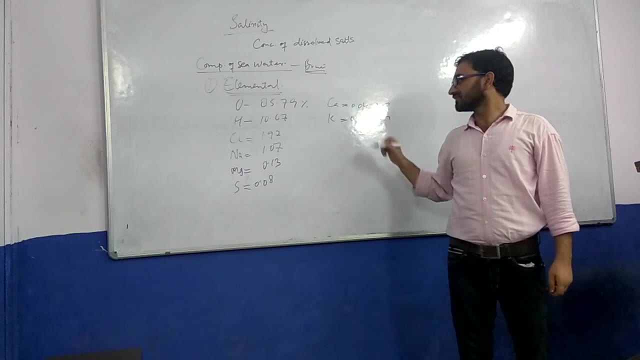 0.03%. What is your name? My name is Madhuri. Yes, Manurag Manurag. Is this more or is this more? 0.40.. This is 40.. This is 38.. Oh, sorry. 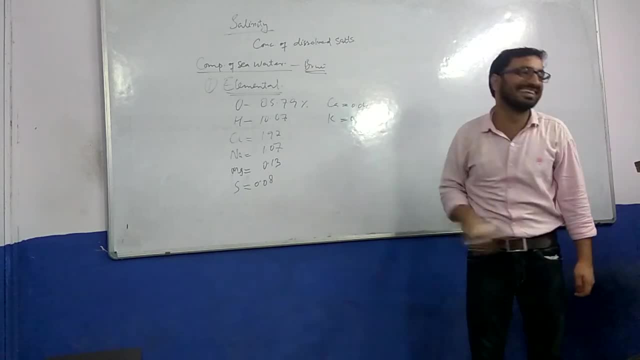 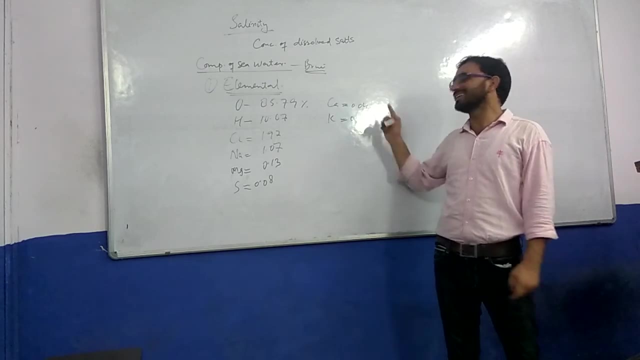 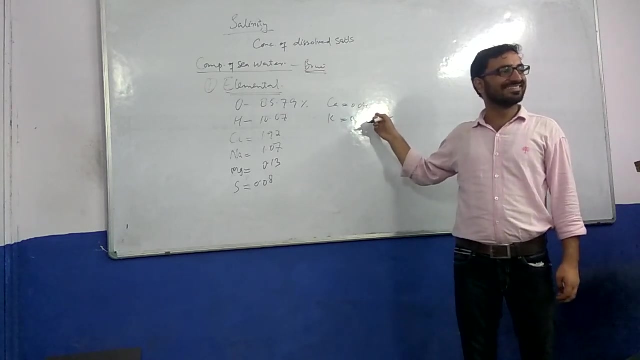 Keep it as 4.. When I wanted to ask, you answered: This is 38 and this is 4.. What is more, Which one? Calcium, Calcium? Why Calcium? It is этот. Yes, That is Tommy's question. 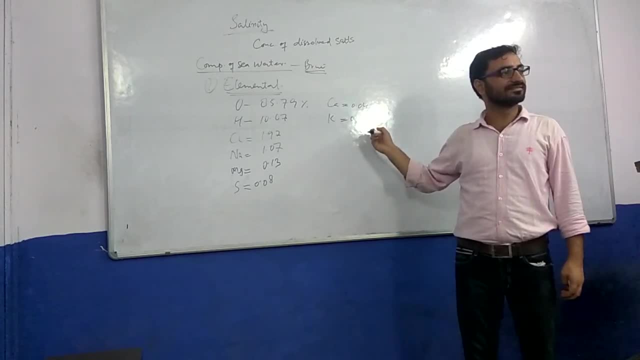 That is 4, this is 38. This is 38.. Also less, It is still less. That one is 38 and 38 makes it less. Yes sir, No sir, If it is 38. Then this is zero. 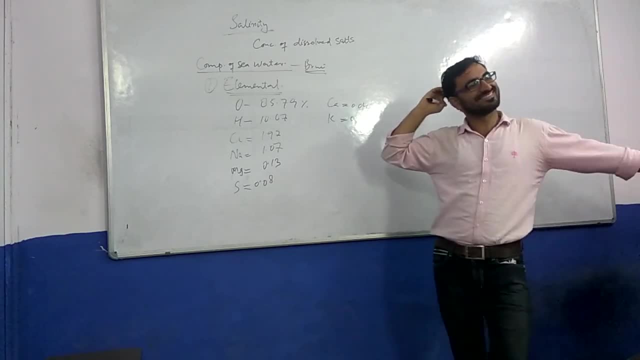 Then it has become 0.. Tell me unes, Yes, nuances and advantages. You say it is more for this or that. Yes, sir, This, What does this mean? Iniration, What is this? Calcium powders. 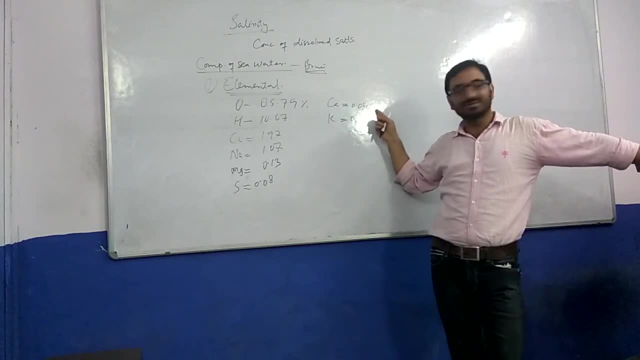 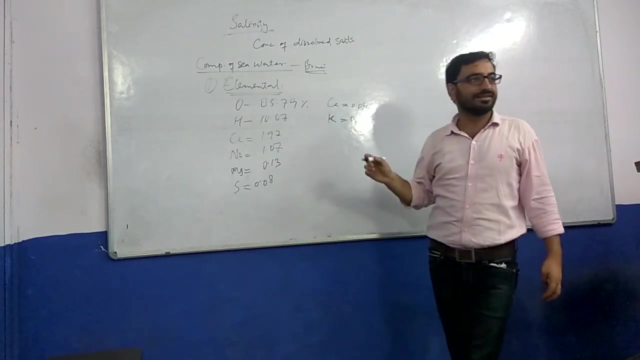 Calcium? Yes, 0.00%, 0.04.. Calcium is more Venka. what is more Calcium? Why not potassium? This is 38,, that is 3,, that is 4.. Okay, So then there is always one element which we call. 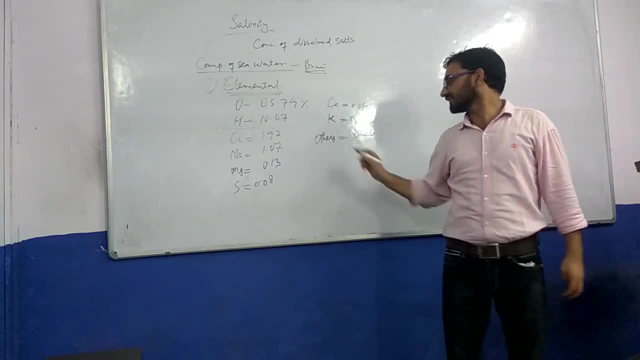 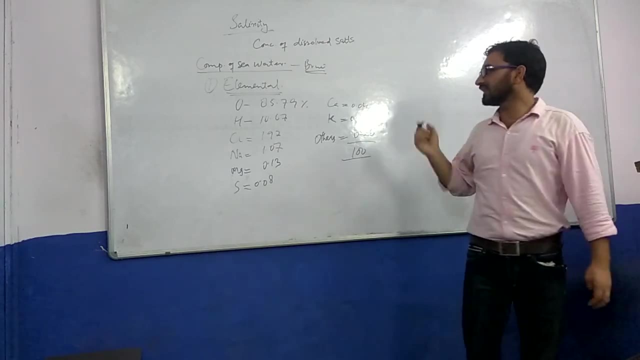 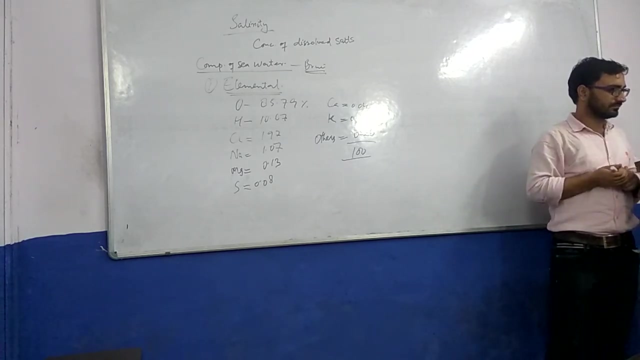 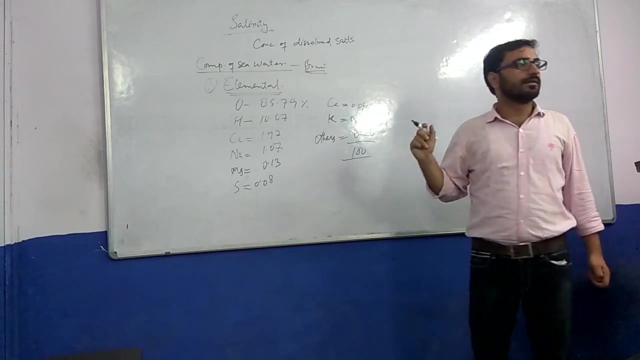 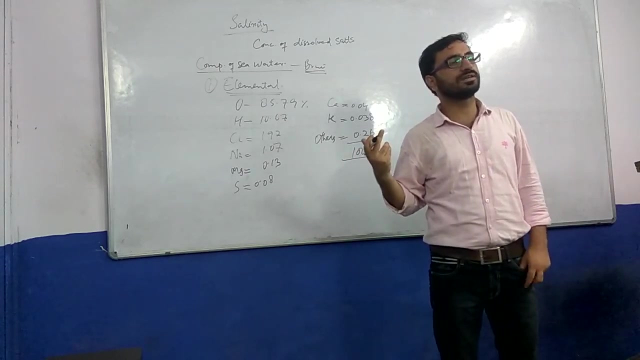 others. That is 0.26% and total you will get something around 100.. Okay, so this is the element of composition of the sea water. Yes, but if you see, why talking, Tell me. ask me Now if you see there are two divisions. 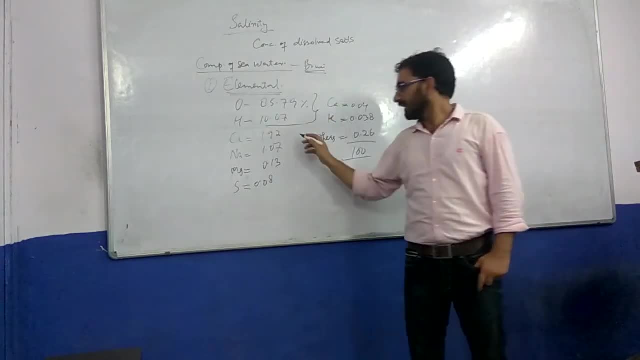 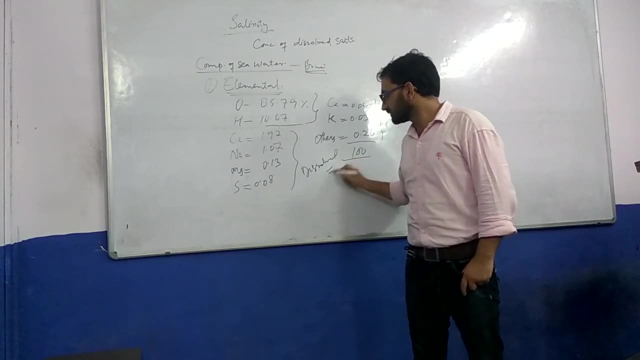 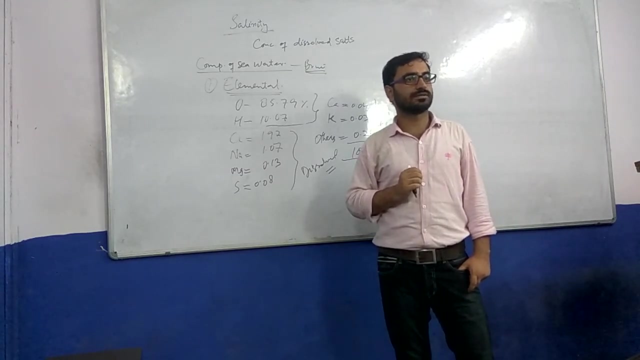 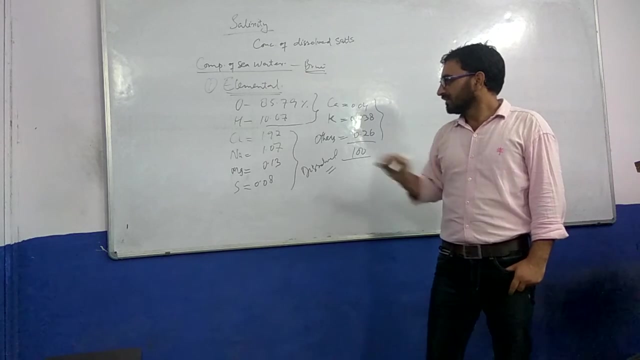 This oxygen and hydrogen is something different And this is different. This is actually dissolved material. This is dissolved material. This is dissolved material, Is it? This is dissolved material And if you look at the dissolved material, this chlorine is around 55%. 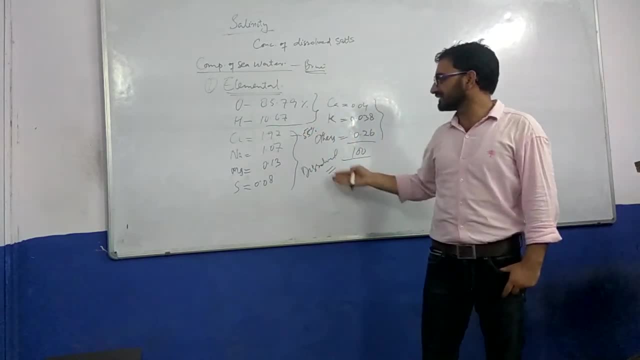 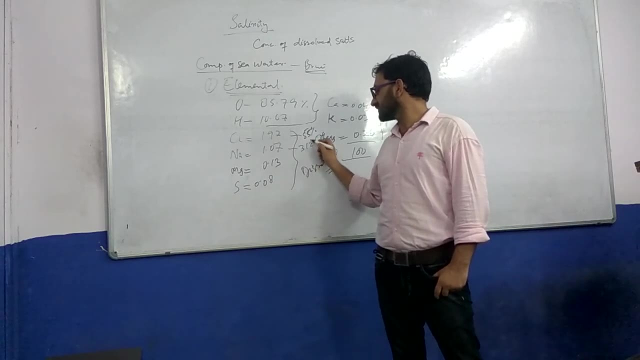 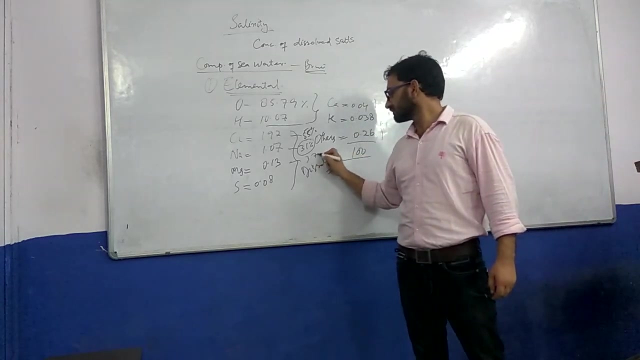 Out of chlorine, sodium, magnesium, sulfur and calcium. there is chlorine, which makes 55%, And sodium makes something like 31%, And then there is magnesium 3.7%, And then there is magnesium 3.7% And sodium makes something like 31%. 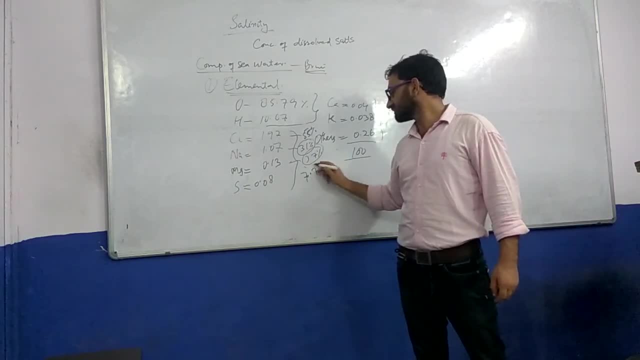 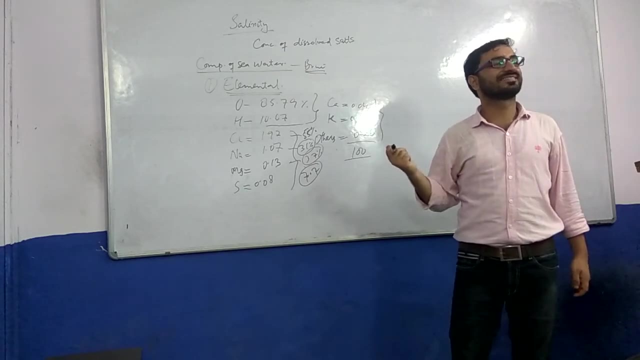 And then there is sulfur which makes 7.7%, And then there is sulfur which makes 7.7%. Now Fraenker will give the answer Now. tell me the answer Now. this is 0.13, this is more. 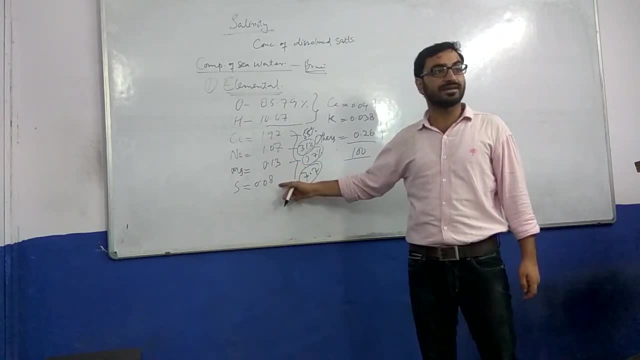 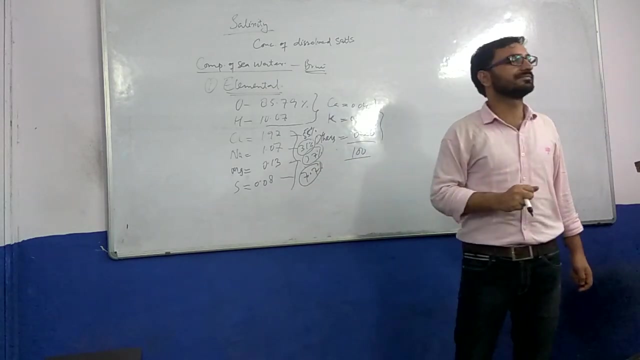 This is 0.04, 0.08,. this is less, But what happened to its percentage? This is 0.13,. this is 0.8, more than 0.13.. I am showing 7.7 points of this. 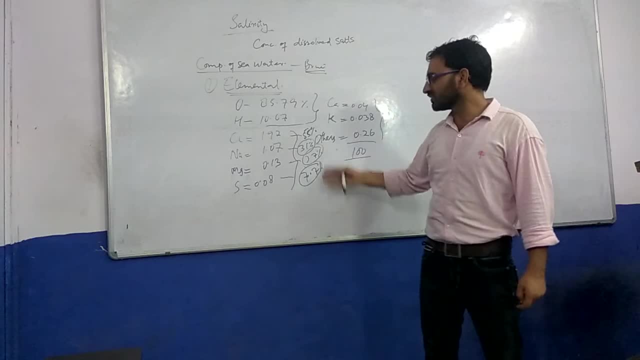 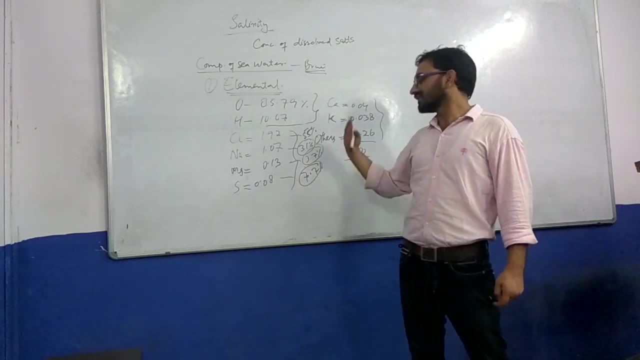 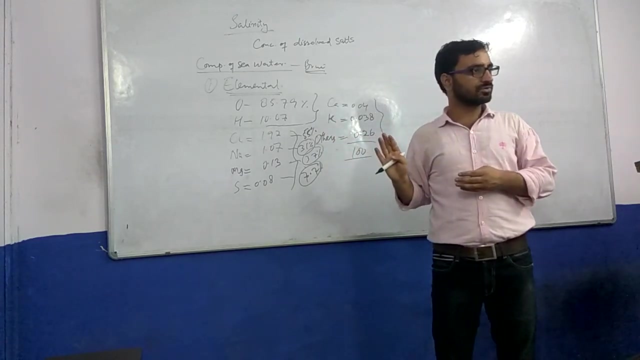 Tell me. You have to keep in mind that Chlorine is more, Sodium is less, Magnesium is very less, Sulphur is more. Different books still give different data, Please, So in your examination they won't ask you the figure. 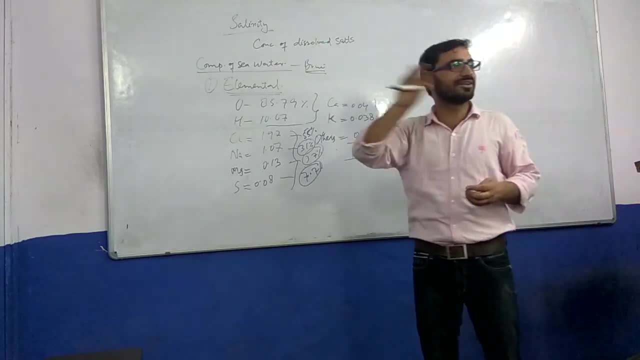 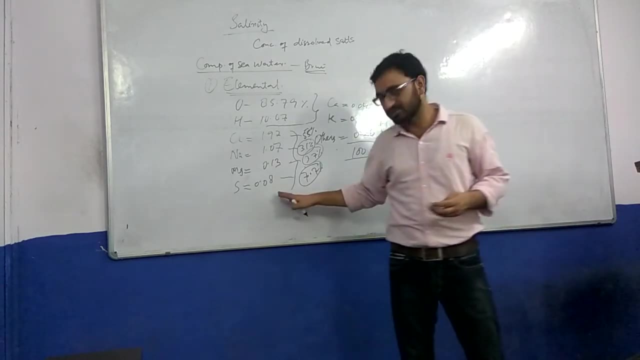 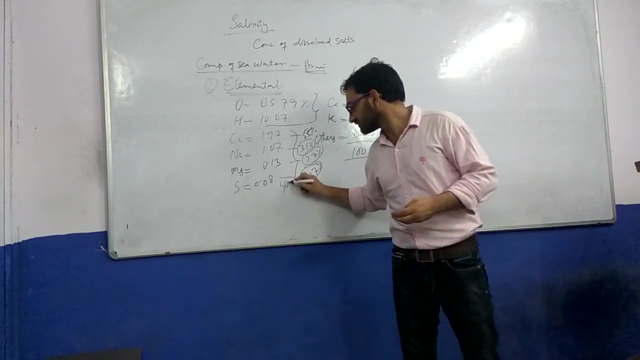 They won't ask you the figure. They will ask if you are increasing or decreasing the order. Now give the answer. I mean, is this possible? Yes, Actually, this 7.7 is not S, It is SO4.. SO4 is 7.7 points. 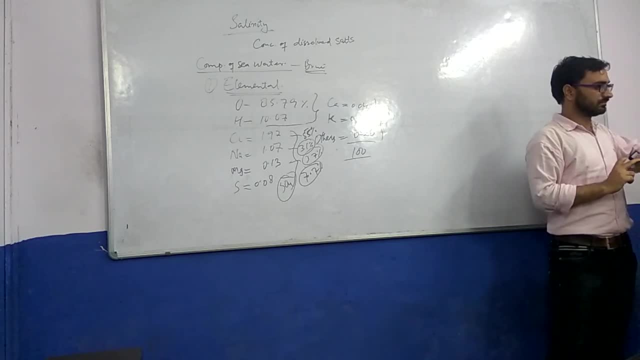 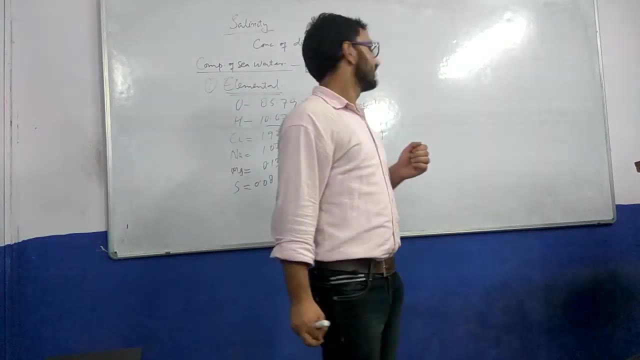 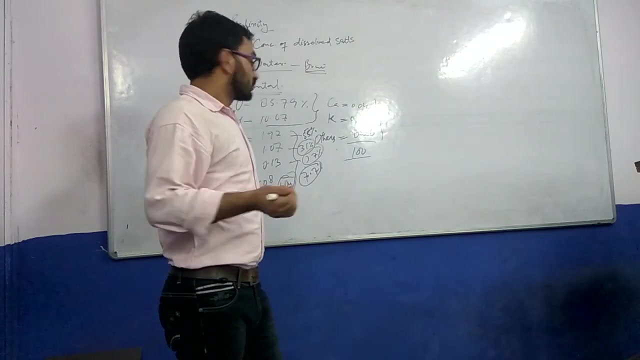 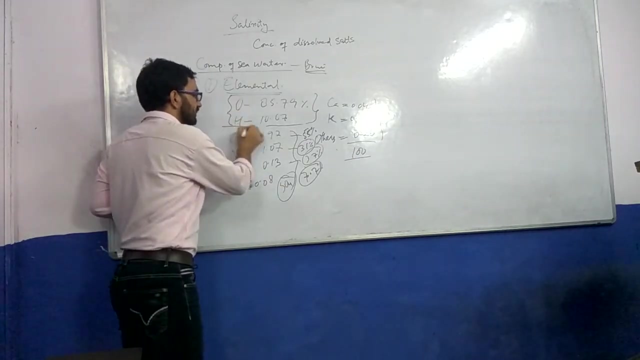 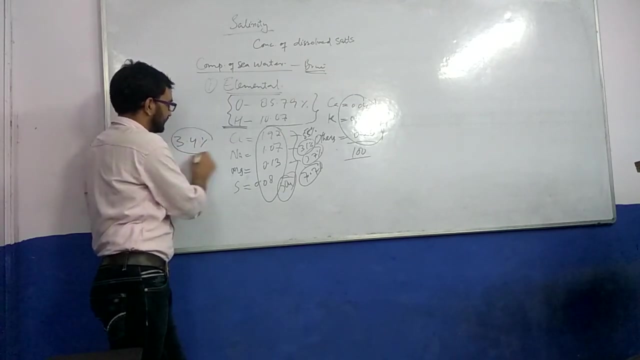 quantity of this Here in the corner? What Animal level? Elemental percentage. Yes, we will discuss that some other time. So Look here, don't talk. Target this Oxygen and Hydrogen, just target it. If we add this as a percentage, what I am getting is it is somewhat between 3.4 percent, something like this. 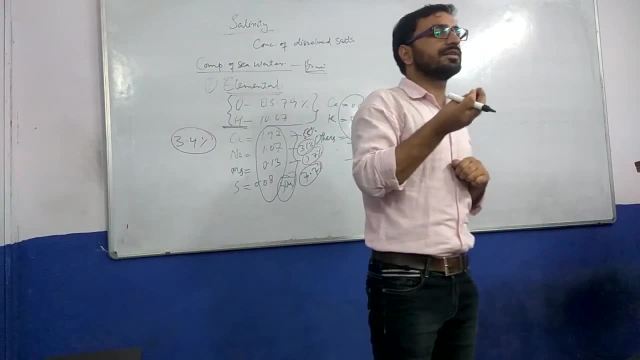 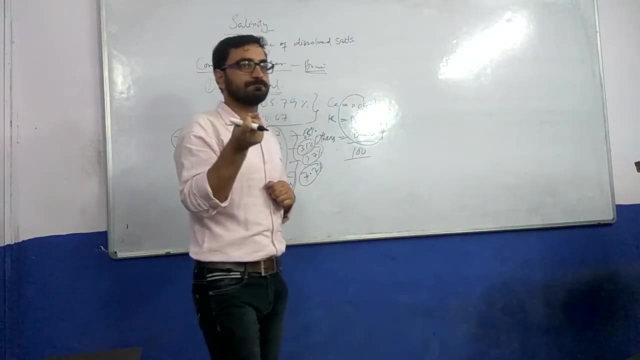 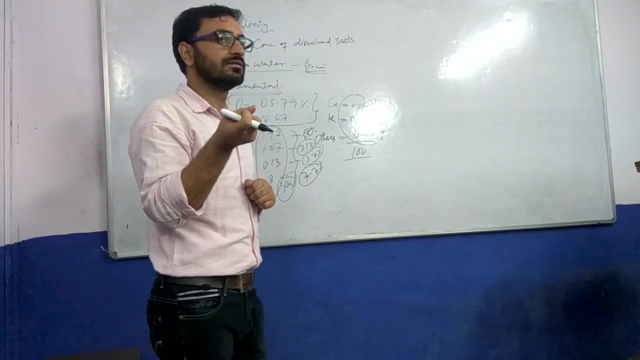 3.4 percent. So 3.4 percent is what It is, the salinity, 3.4 percent is the salinity. But question hai. No, sir, I was talking to him and he was saying that if we add other machines, it will be 0.06, not 0.06.. 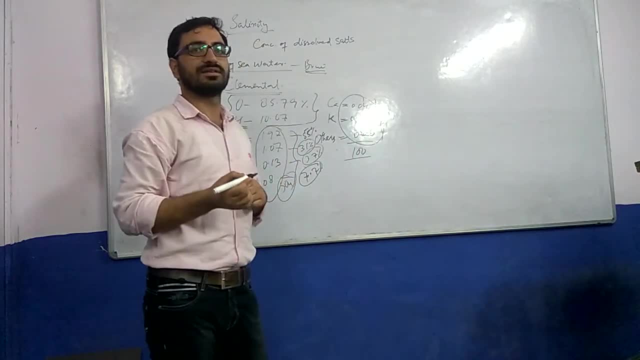 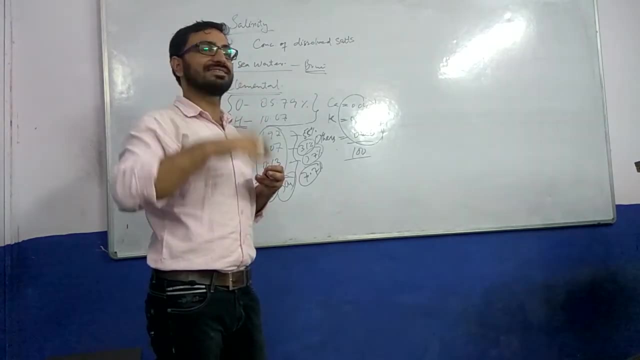 Yes, so add 0.05,, 0.06,. what is the big deal? You are following all these things. In addition, subtraction: where is wrong? where is not? what you have to learn, you don't learn. 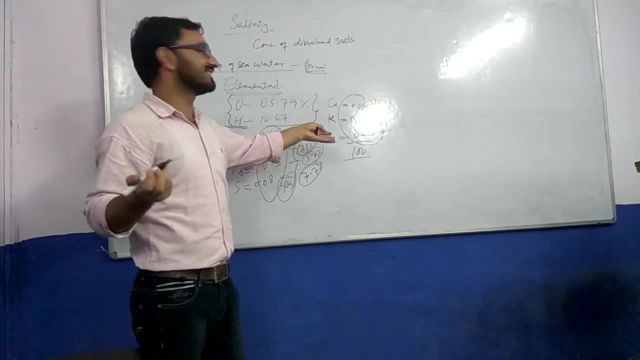 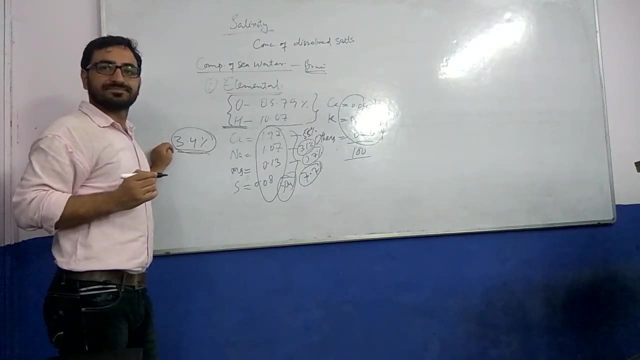 Where to add 0, forgot to add where to add. there are small things. I want to teach you something else. you learn that. So salinity here is 3.4 percent, Here we have 3.45 percent. 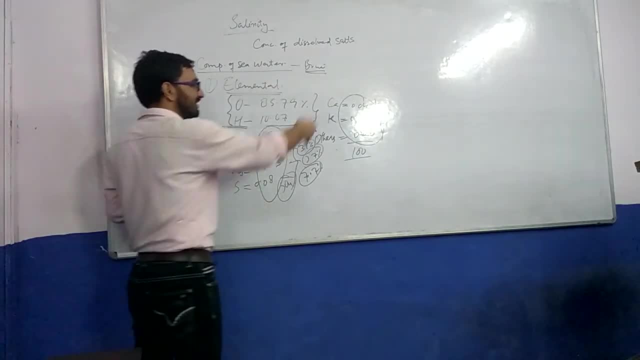 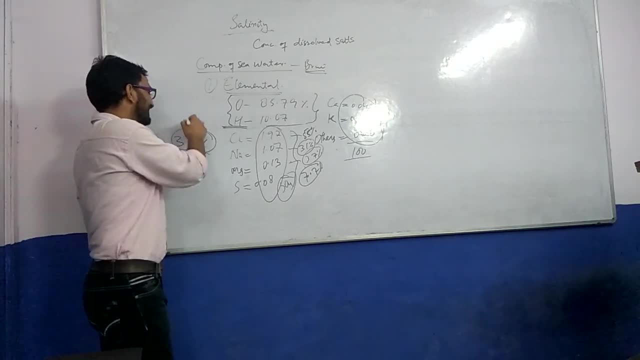 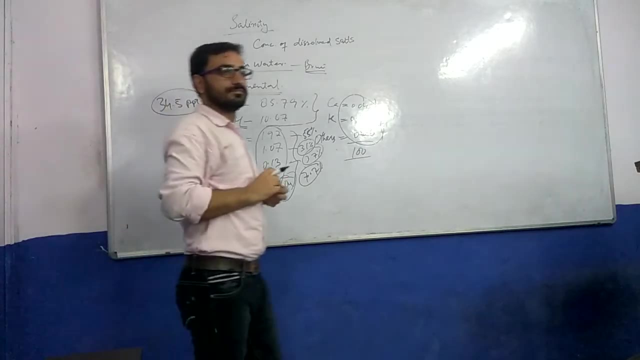 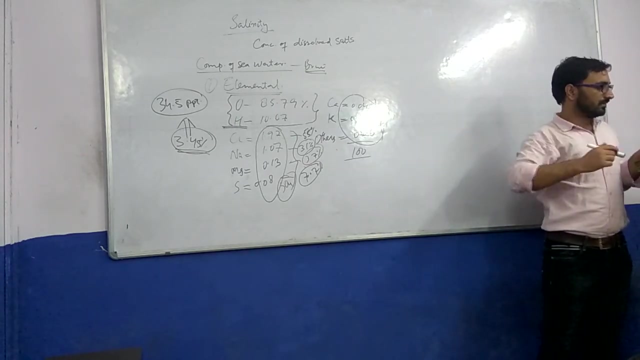 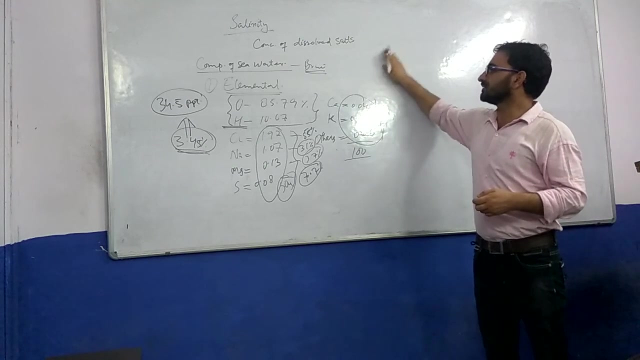 So we usually write it in PPT, So we make it like 34.5 PPT, 34.5? How it is- 34.5 PPT. Let us see the- you know- solid composition, elemental composition. let us see the solid composition. 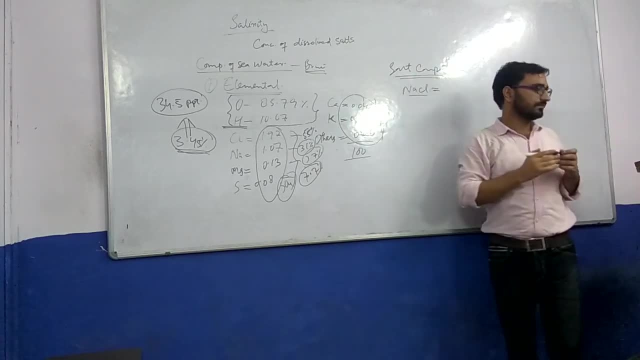 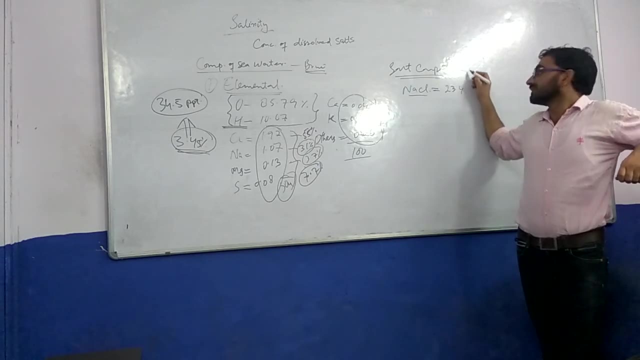 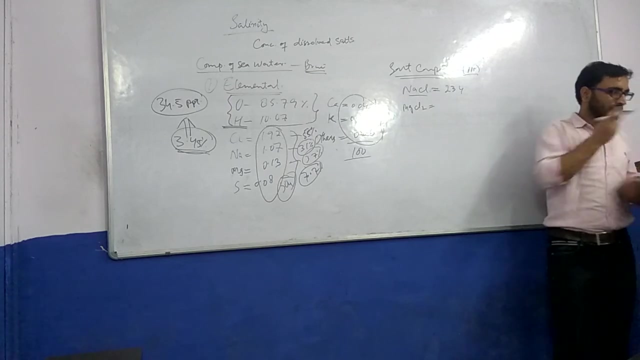 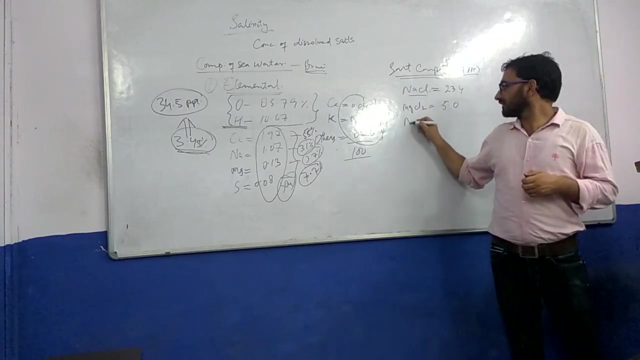 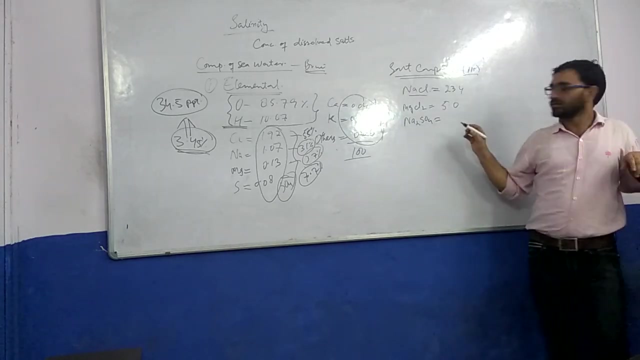 First of all write NACR, NACR, look 23.0.. But what PPT, 23.0 PPT. Then look at MgCl2.. MgCl2, 5.0.. NACO, SO4, sodium sulfate, 4.0 PPT. 3.0. 4.0.. CaCl2.. CaCl2. 2.0. 2.0.. 1 ppt: 1.01.. KCL: 0.7.. Others: 0.8.. Total: 34.5.. This is the salinity. 34.5 is the salinity. 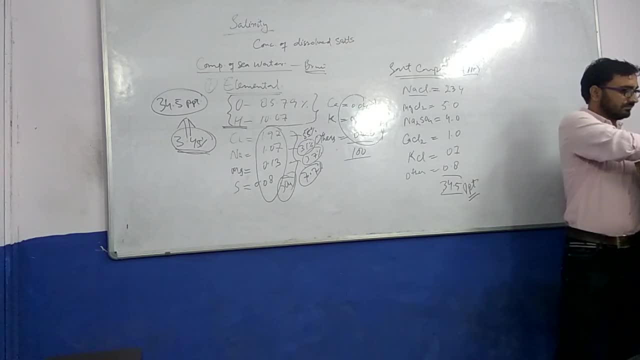 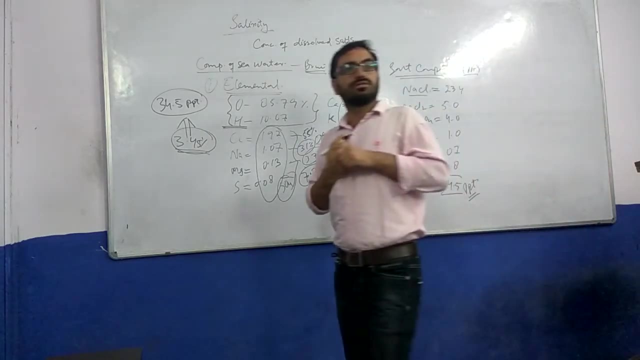 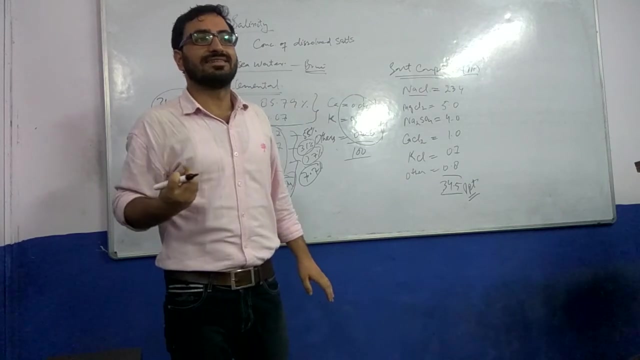 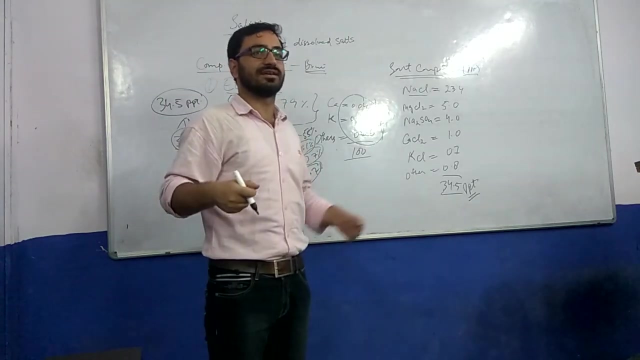 Now just keep a little bit of data. Now the point is that where do these salts come from? Where from this salinity comes? You make vegetables at home and you add salt to it. Who adds salt to this, Huh? 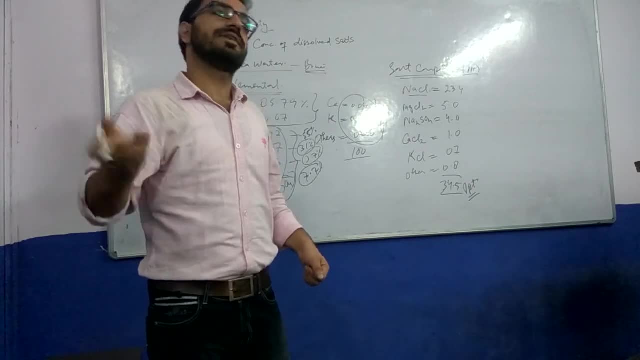 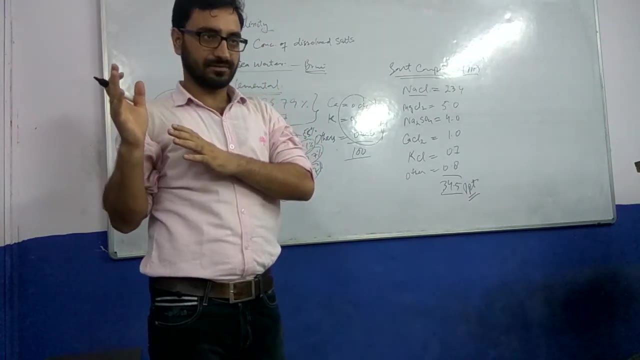 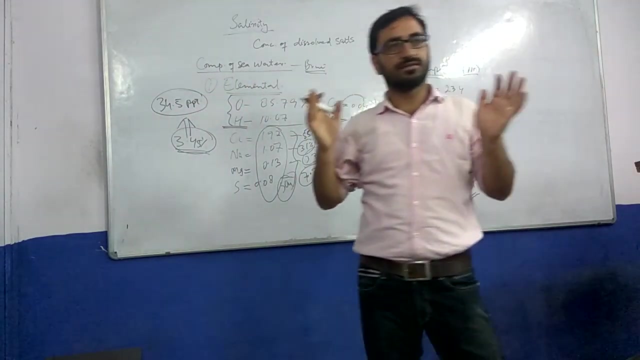 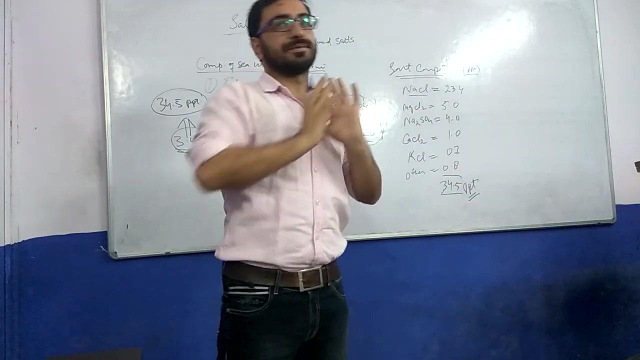 Where does it come from Weathering right Weathering and erosion Sources: land Weathering and erosion of continents. Sources weathering and erosion of continents: Mountains, rocks, soil. From there, the salt erodes and goes into the ocean. 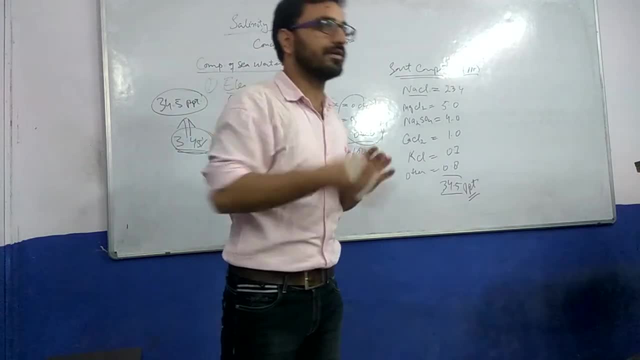 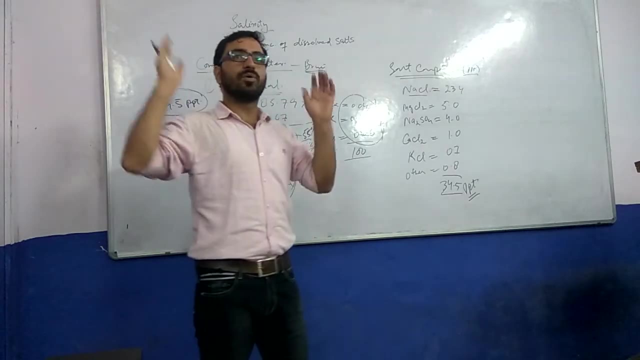 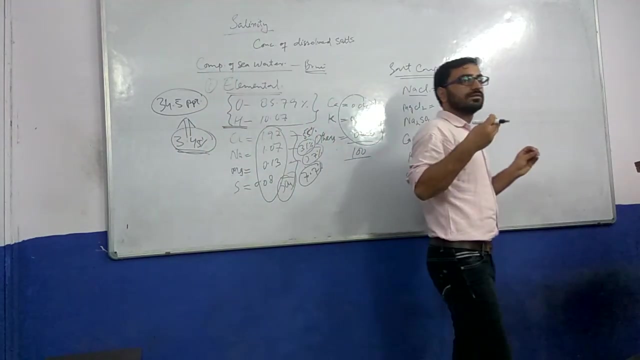 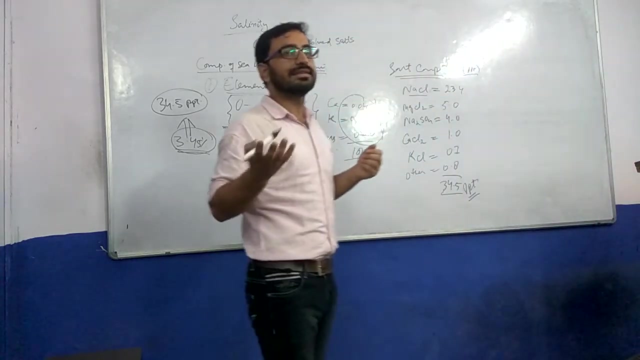 Most of it Through the river water and little bit through- you know, aeolian processes, Through the wind, through the glacier, But most of the salts that go into the sea or ocean is through water. Water is the transporting medium. Let's see, Let us see it. Is it possible? 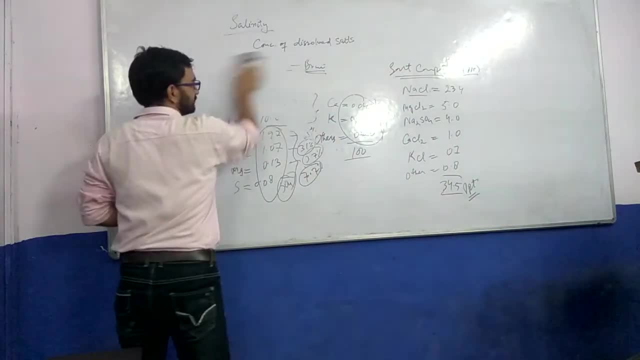 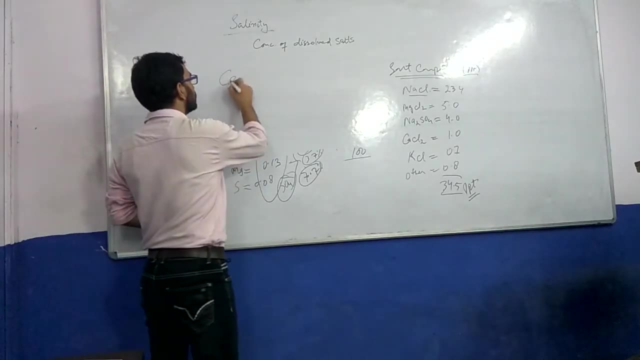 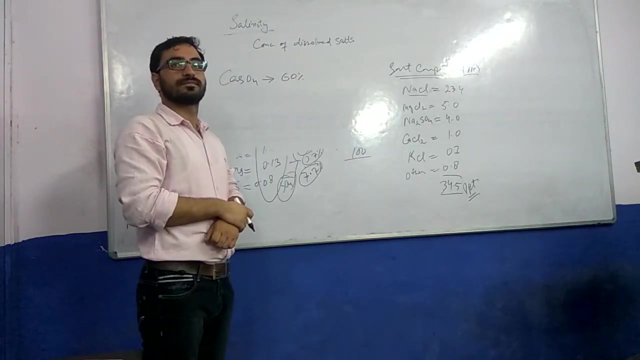 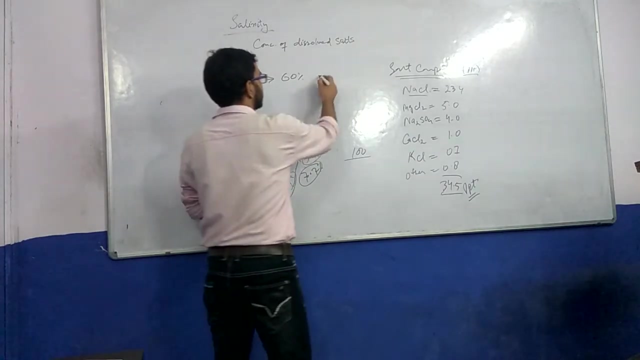 Let us see it, Let us see it, Let us see it. When this river water has been seen, it has been seen that CaSO4 is 60%, And when CaSO4 was seen in the ocean water, it was just 1.5%. 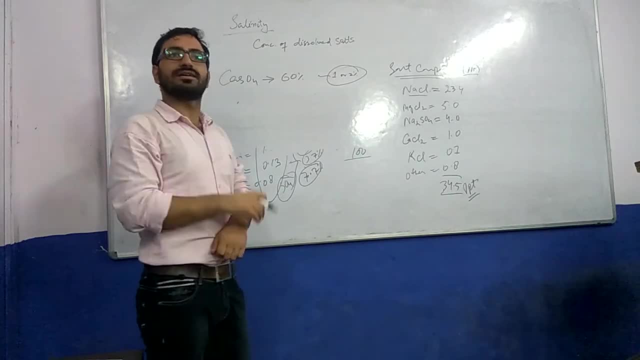 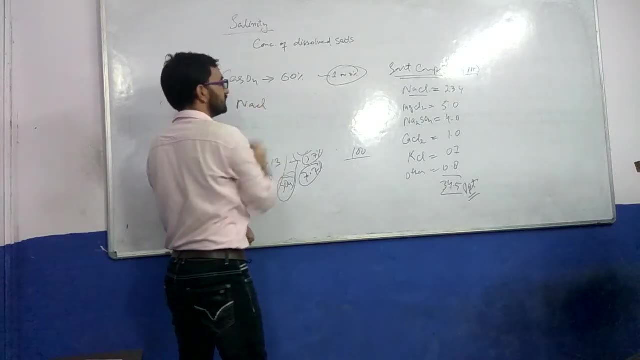 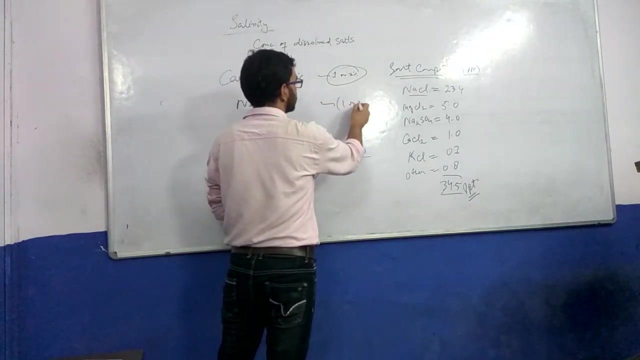 Aeolian. Aeolian Aeolian: What is dominant in the ocean? NACL: Nearly 55 to 60%. When NACL was seen in the ocean water, it is not in the river water, It is very less. 2 ppt. 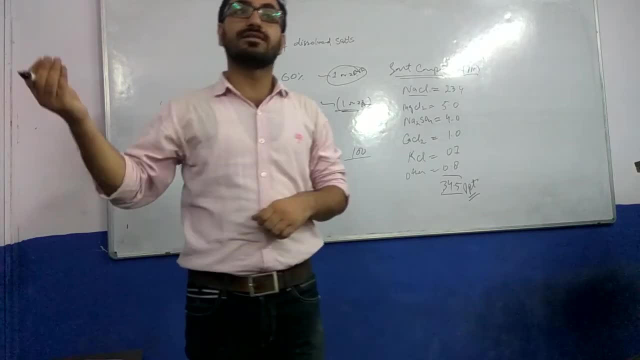 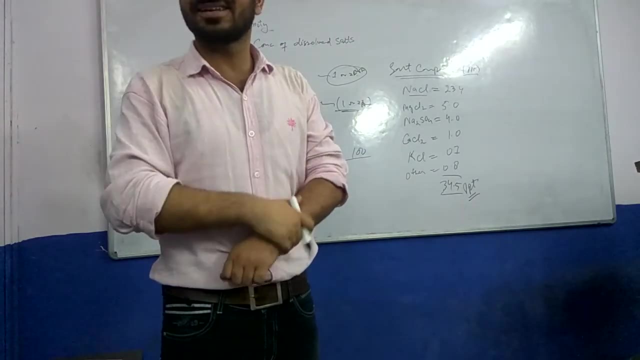 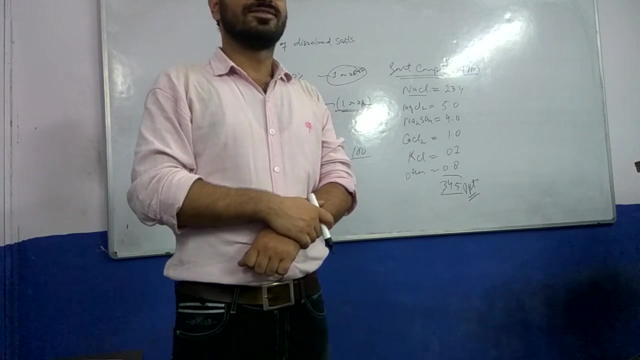 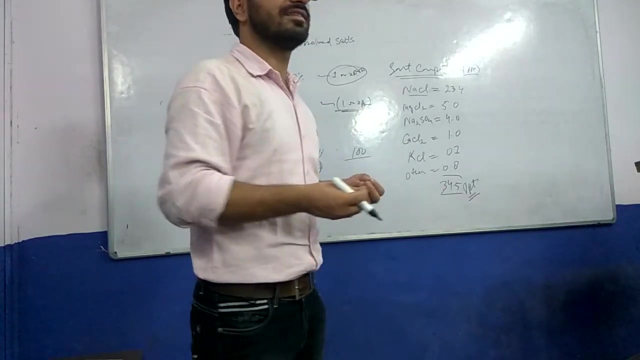 Sir, you are saying that it comes from the river, But there is no NACL in the river. It is very less. here There is CaSO4 in it, CaSO4. So we are wrong. Right, We say. Books say that salts come through the river. 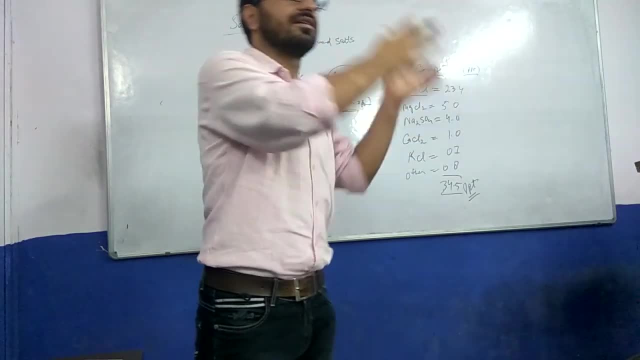 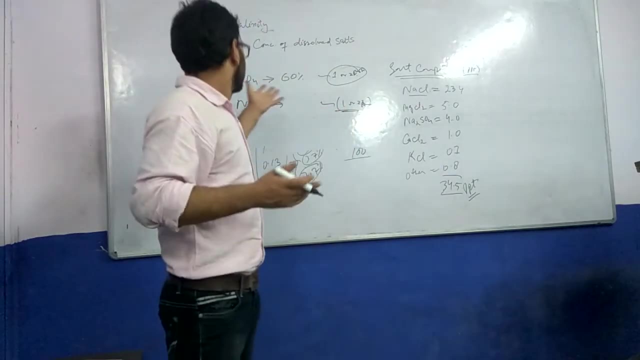 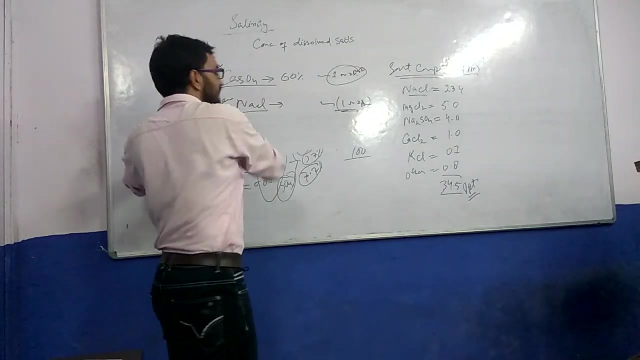 Salt comes through the river water and goes into the ocean. Is it true or false? Is this statement true or false? We have seen the composition of the river water. We have seen the composition of the ocean water. It is contrasting, it is different. 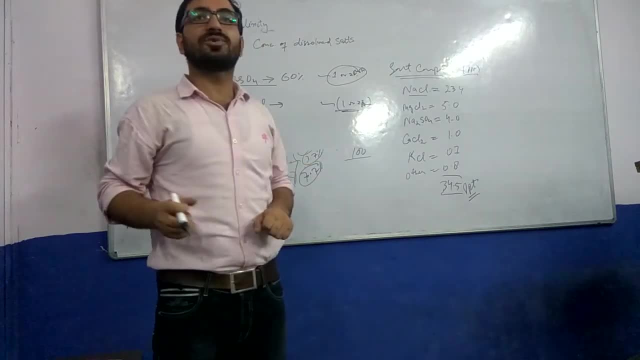 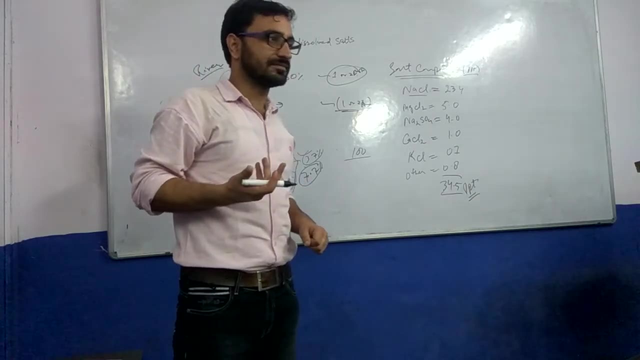 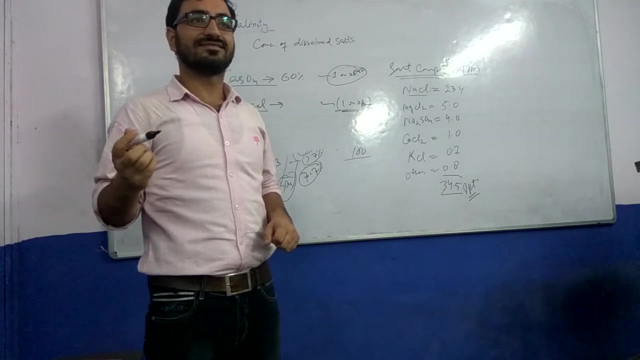 Here, NACL is more here, CASO4 is more. Now what will happen? It means there is no reversing. Even after telling so much, they say: there is no reversing Then. So here comes the another point, another concept to what we call Residence Time. 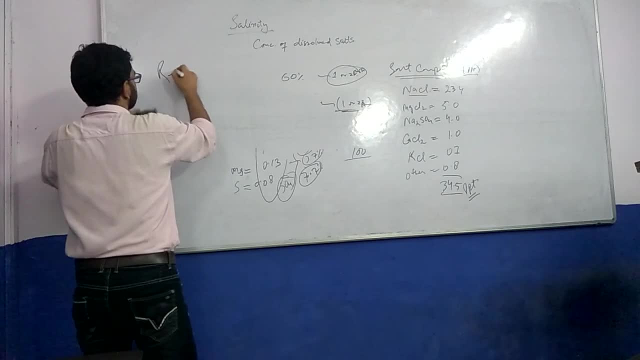 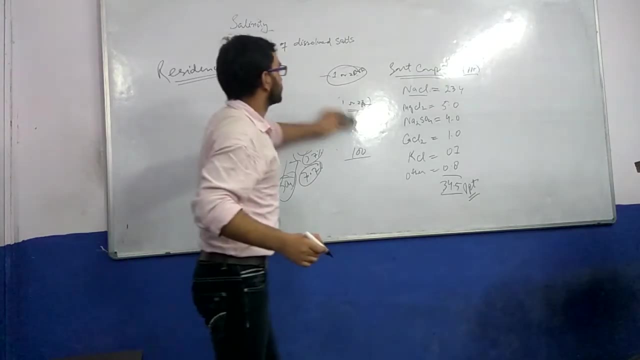 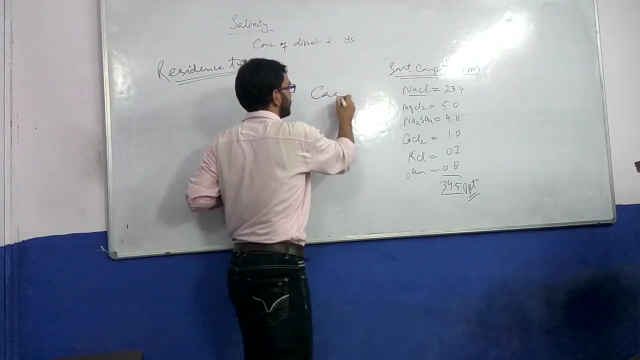 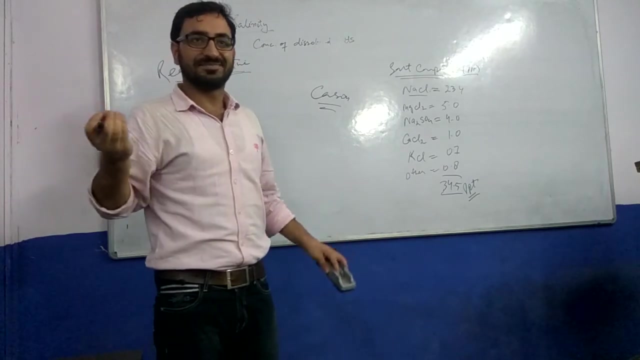 What we call Residence Time. Residence Time: For how long does something live in a place? It is called Residence Time, The SO4 that comes from the river. its residence time is very less. This calcium is picked up by the organisms, So 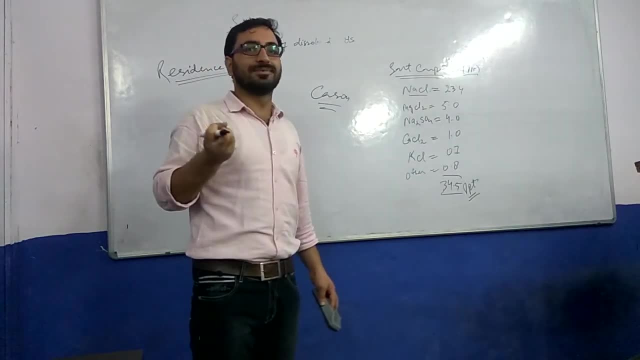 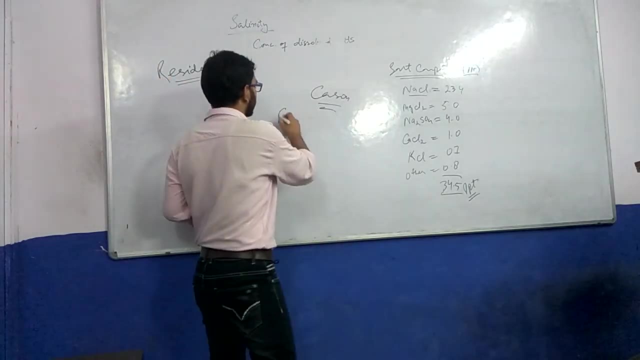 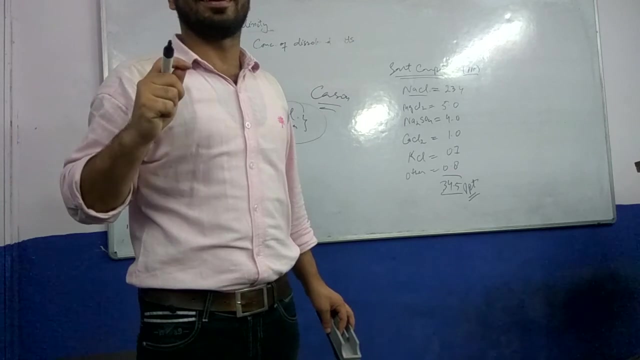 the calcium here is picked up by the organisms. They make their shells because of the calcium, So its residence time is less. The residence time of SO4 and chlorine is the maximum. The residence time of SO4 and chlorine is the maximum. Because of this residence time we get concentration of SO4 in the ocean water. 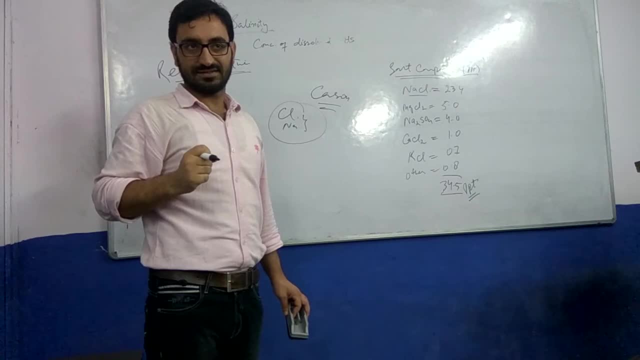 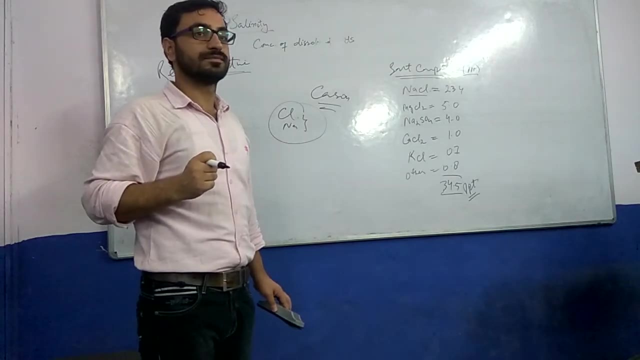 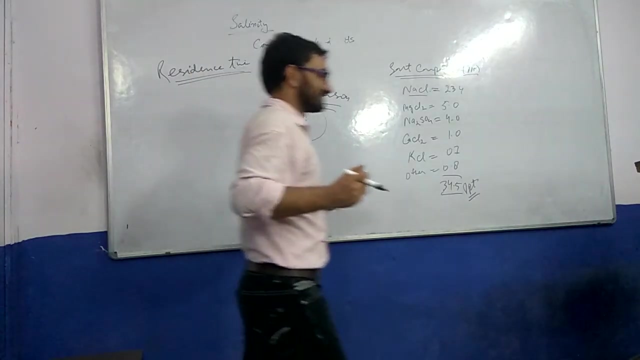 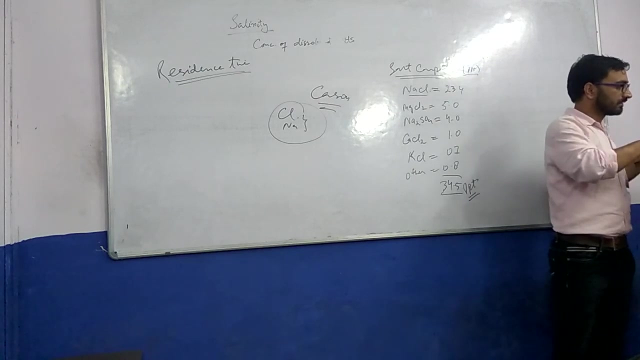 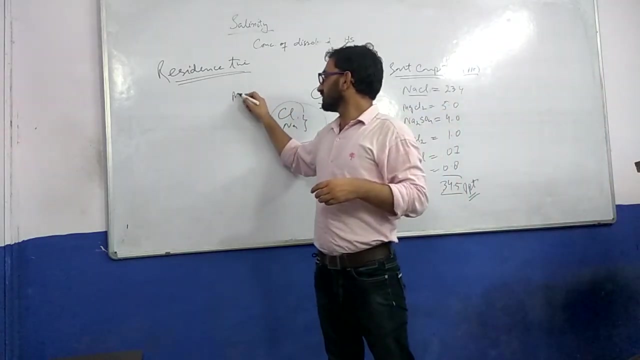 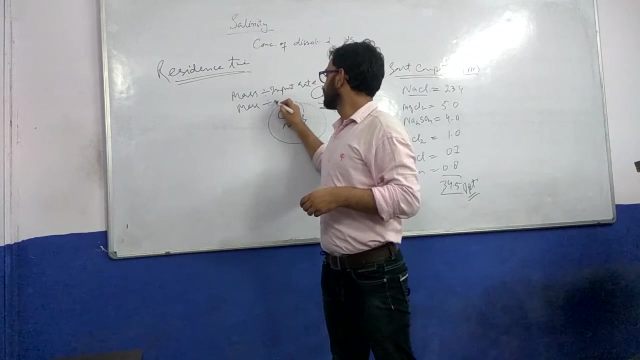 Because of this residence time, we get concentration of SO4 in the ocean water. What is residence time? It is the ratio of rate of input and output, rate of input and total mass divided by input input rate, or total mass divided by output rate. 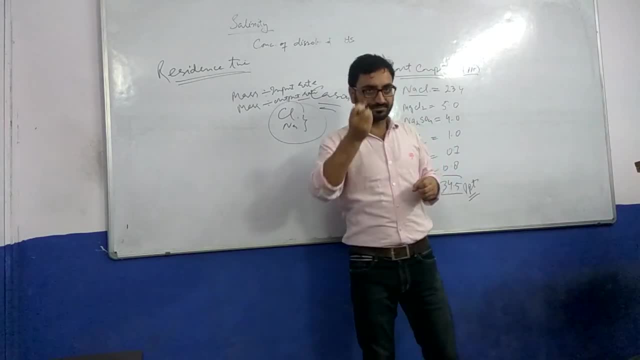 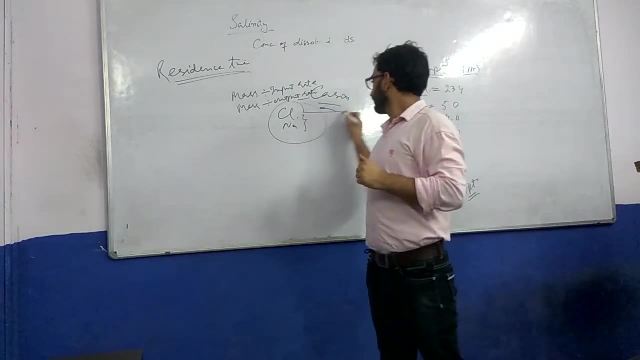 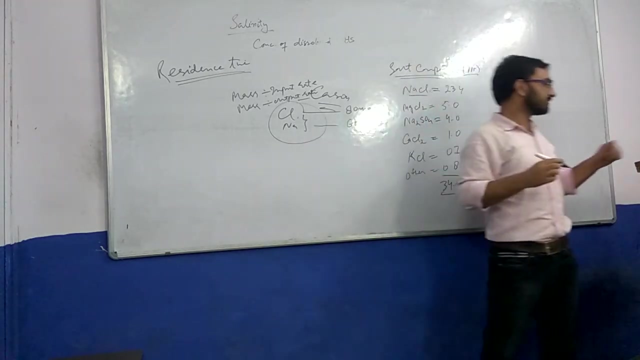 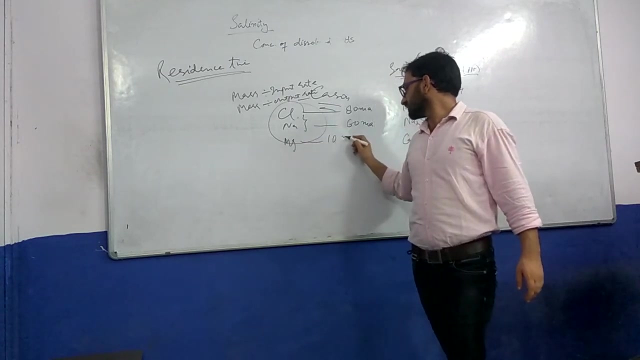 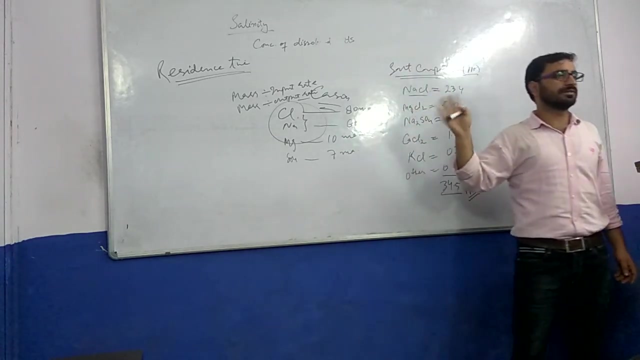 Anyway. so write this. You write the residence time of chlorine. Chlorine is 80 ma. Sodium is 60 ma. What is ma? Magnesium is 10 ma. SO4 is 7 ma, Always. there is a question about residence time Always. 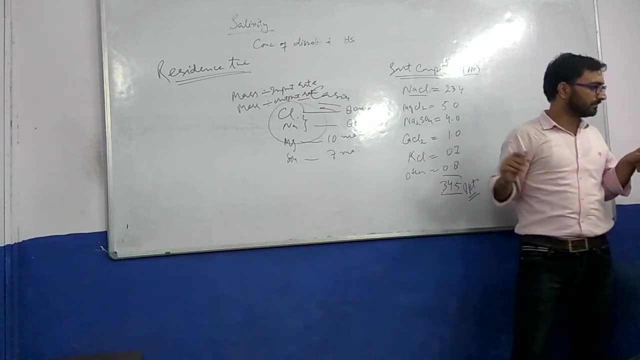 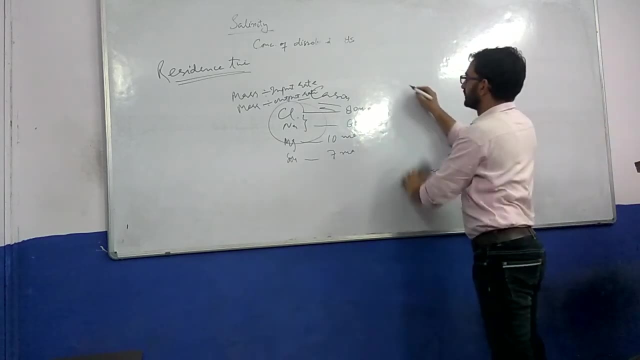 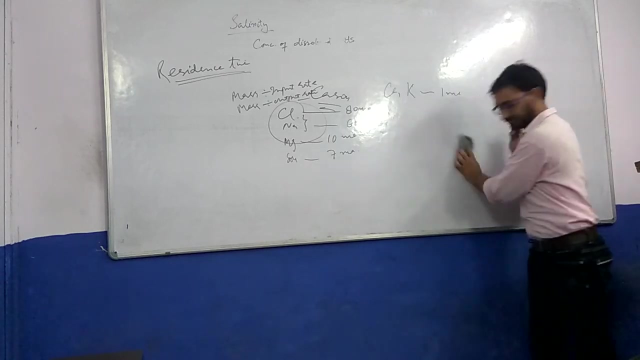 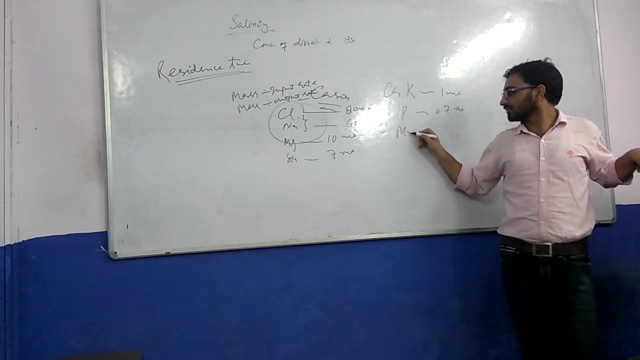 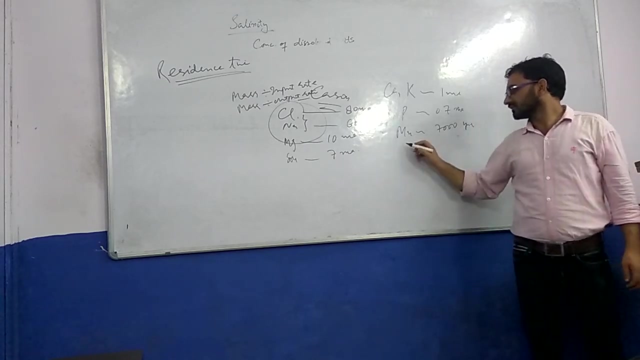 Calcium is 1 ma. Calcium, or potassium, is almost 1 ma. What is magnesium? Magnesium is 0.7 ma. What is magnesium? Magnesium is 7000 years. What is zinc? 5,000 years. What is zinc? 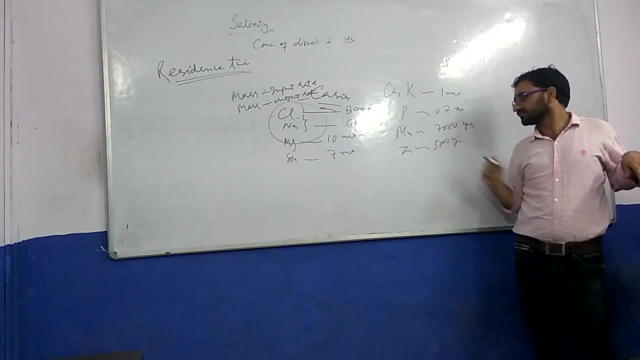 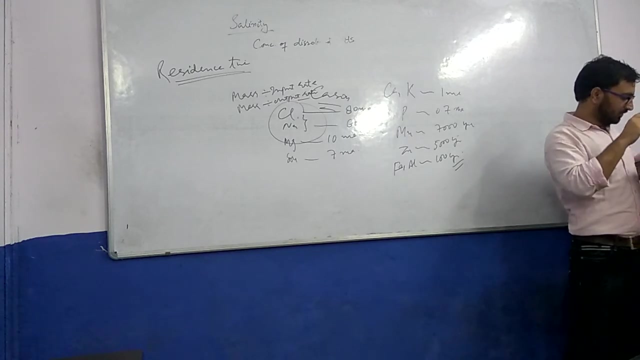 5,000 years, 5,000 years. What is iron? 5,000 years? quasar, quasar, quasar, quasar. What is iron iron? iron 1 ka? They used to ask the increasing and decreasing water. 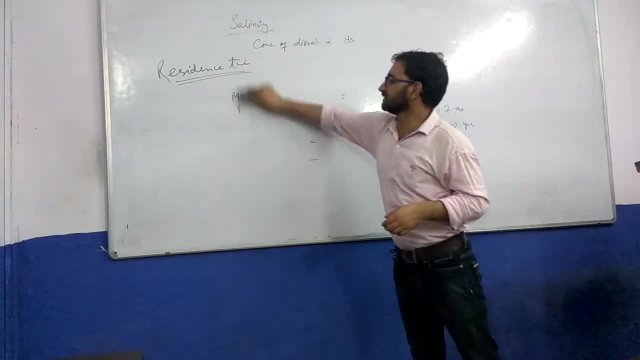 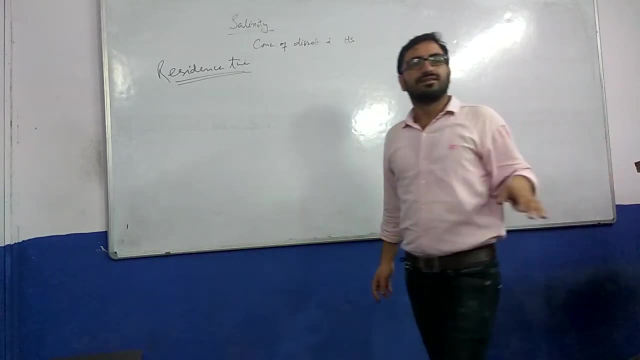 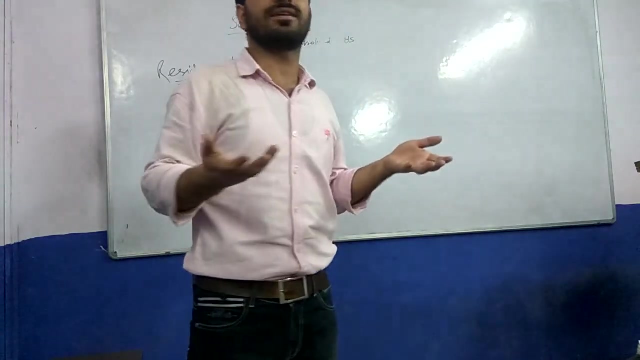 They used to ask the increasing or decreasing water of residence time. So, Sir, Chlorine and Sodium have more residence time. Chlorine and Sodium have more residence time. Calcium has less residence time. That is why we get more Sodium and Chlorine in the ocean water. 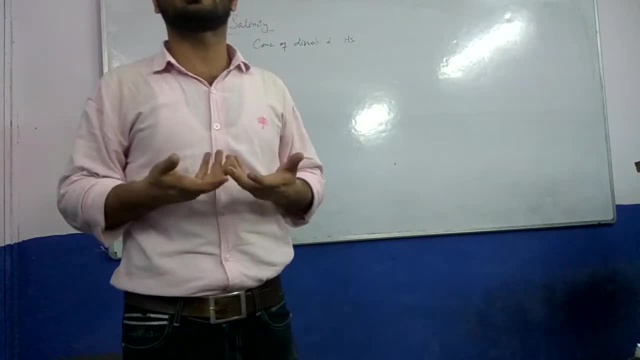 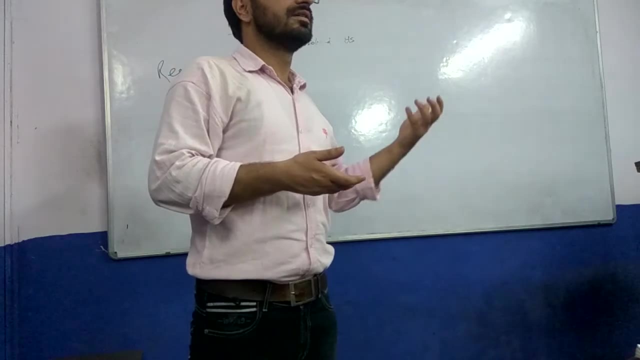 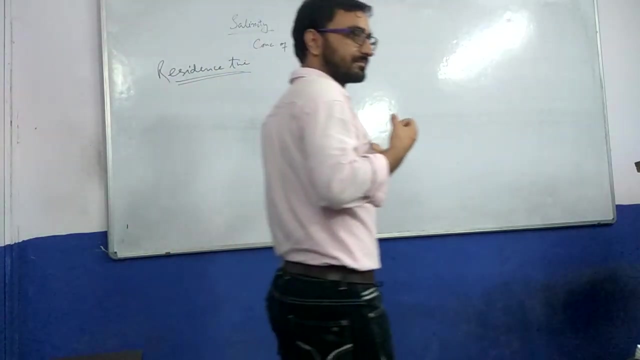 Why? Why we are not getting more calcium there, Although calcium is dominating in the river water. but we don't get calcium in the ocean water because it has been picked up by the organisms. It has less residence time. Sodium and Chlorine has more residence time. 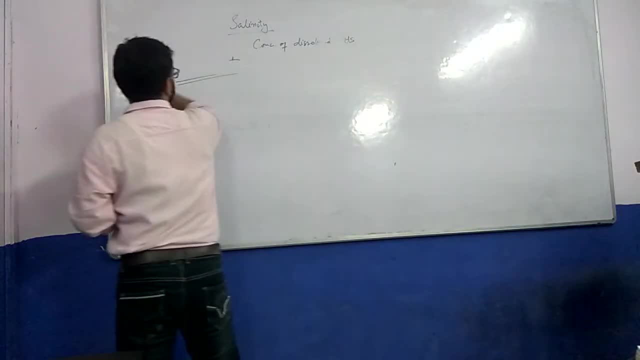 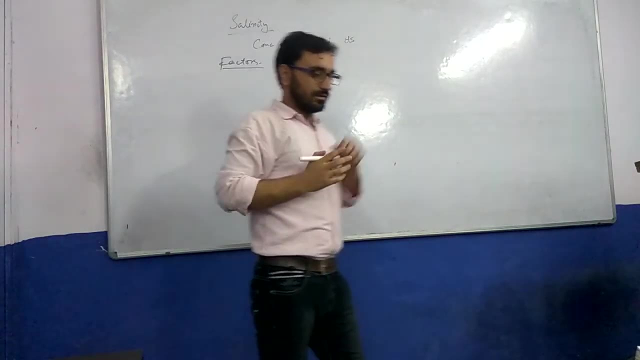 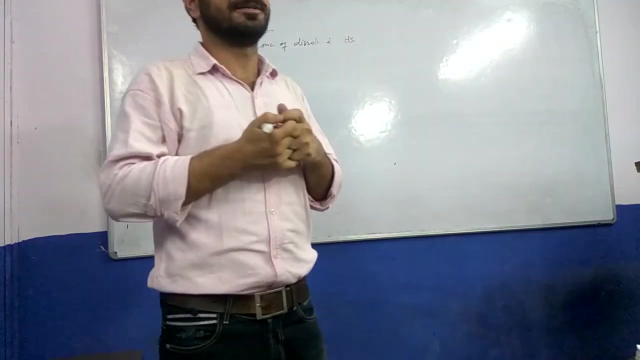 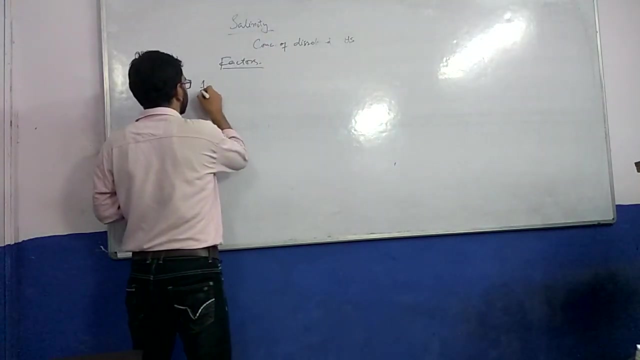 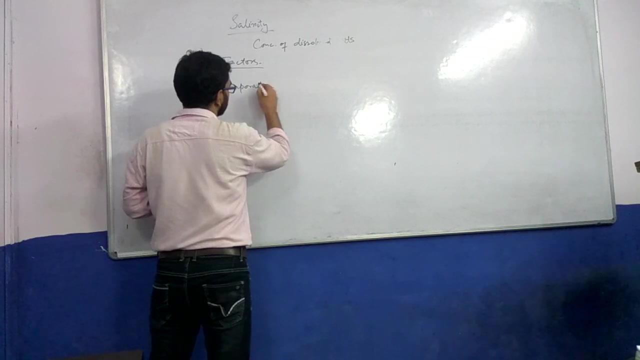 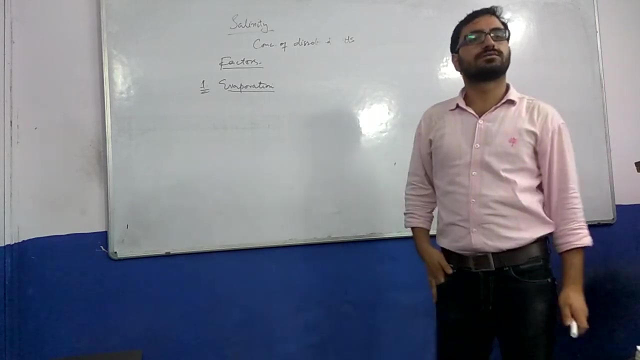 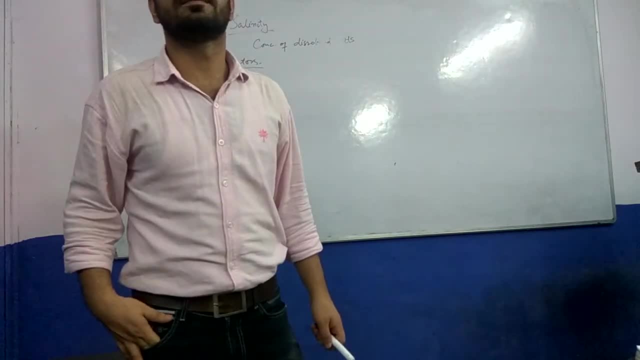 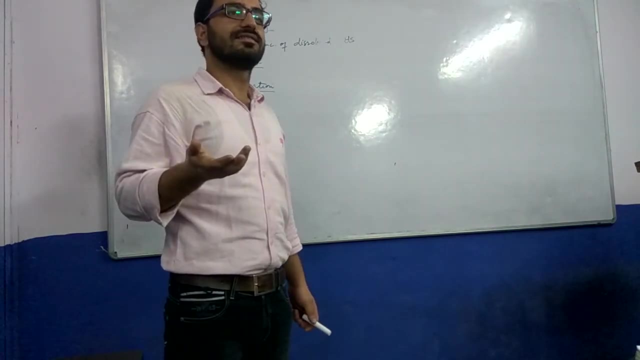 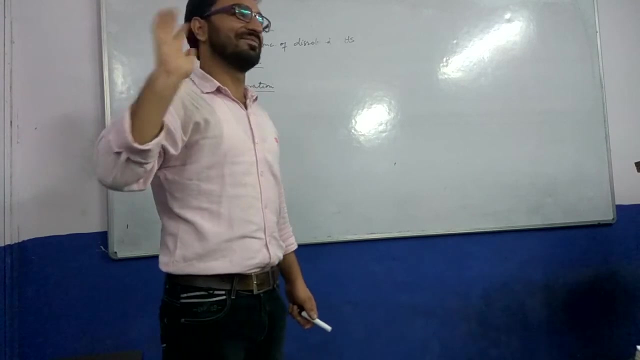 What will happen with Evaporation? Say loudly if you know something: Water is converting into Vapour. Nobody knew about this till today. Just one person is aware about it. In the water it converts into Vapour and it is called the Evaporation. 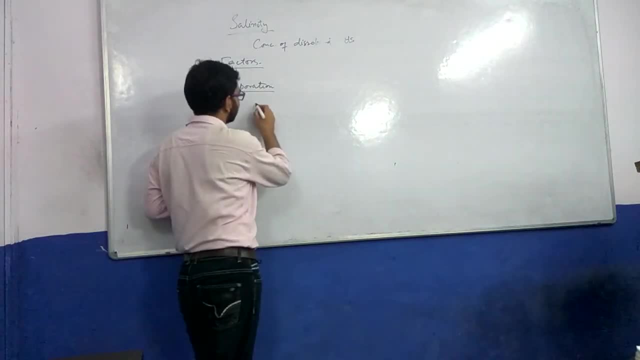 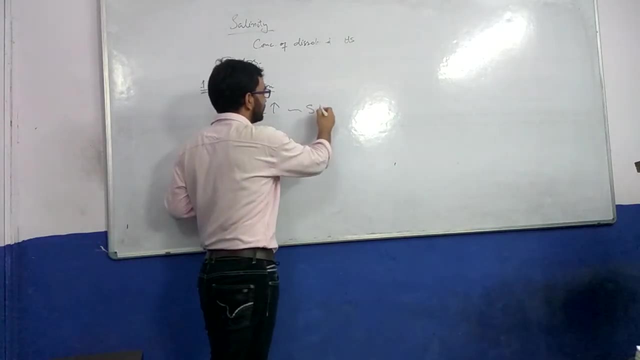 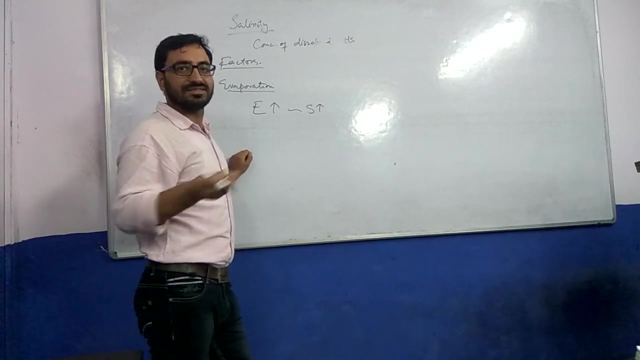 Thank you. So there is increase in Evaporation, evaporation- The salinity will also increase. So evaporation is taught in 6th standard. I am not asking what evaporation is, I am teaching the relation of salinity in evaporation. So if there is increase in the evaporation, the salinity increases. Because what happens in evaporation? Only pure water will go away. Salt will be left over there. If you make sabzi or tea- I said tea because we eat salty tea- You don't drink salty tea, So this example won't work. 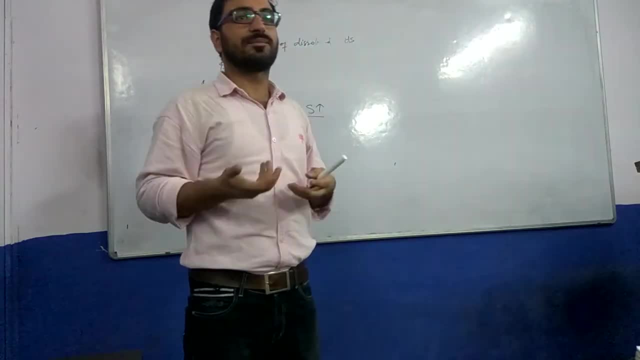 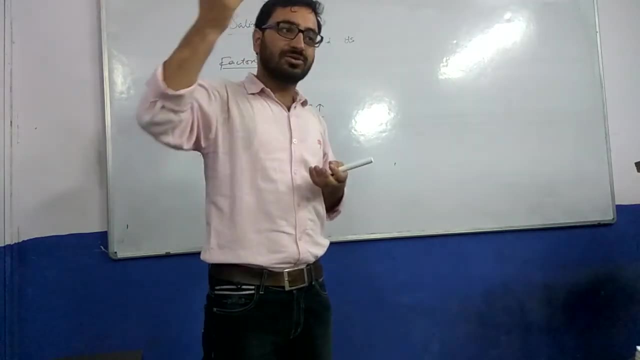 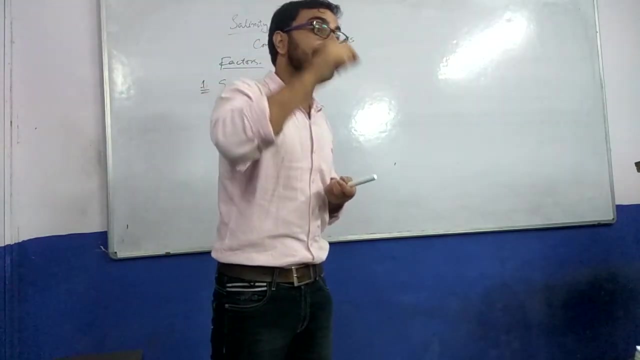 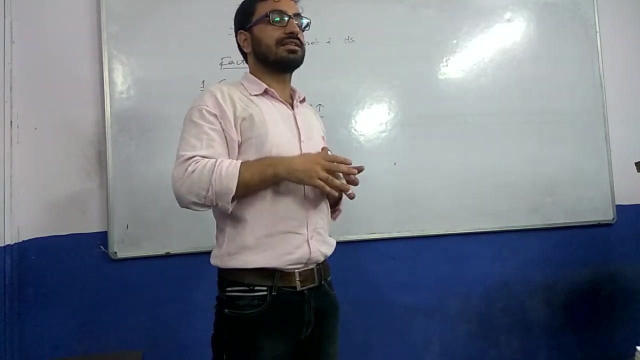 So if you boil the sabzi for a long time, the salinity will increase Because evaporation will happen. Because of evaporation, pure water will go away, So salinity will increase. Concentration of salt will increase. Concentration of salt will increase. Similarly, in tea, the sugar will increase. 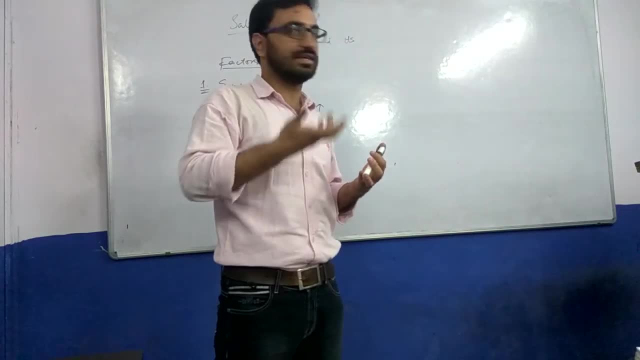 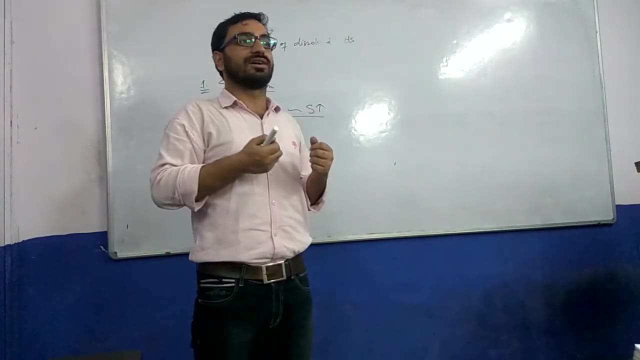 If you boil a lot, there will be a lot of salt present in his or her body. So same thing is the case with evaporation. Where we will get more evaporation, salinity will be more up to that point. Where will be more evaporation. 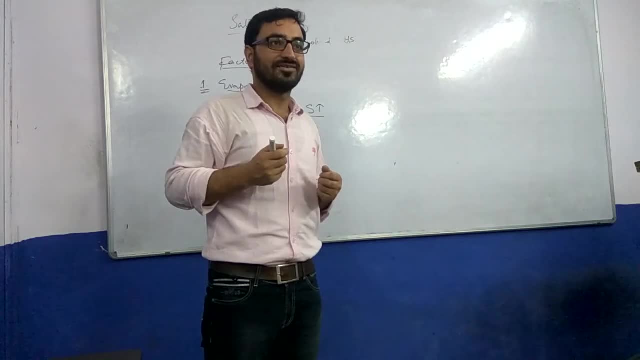 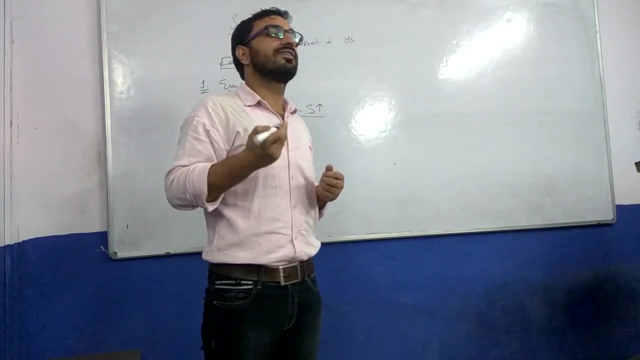 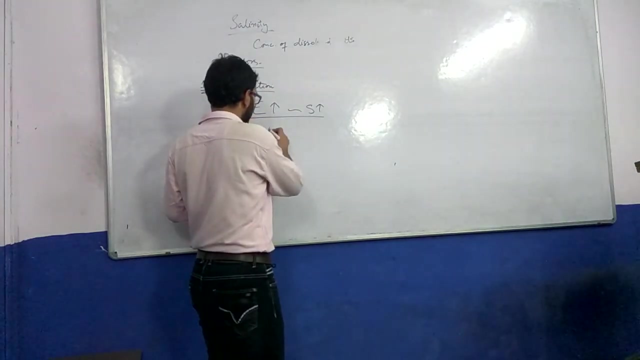 that too, we have studied. on equator, evaporation is more. who has studied? no, who has studied on equator, where evaporation is more: 30 degrees, around 30 degrees. so on tropics, which is usually said, on 20 to 40 degrees, evaporation is more. 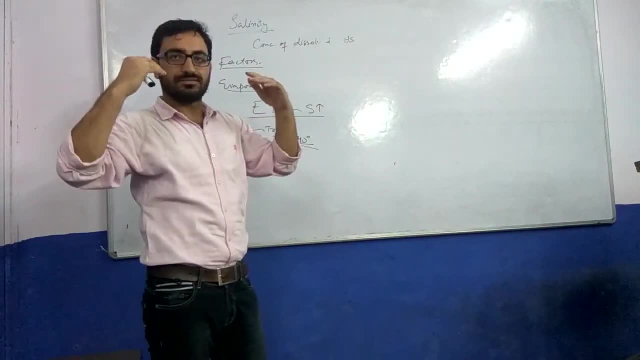 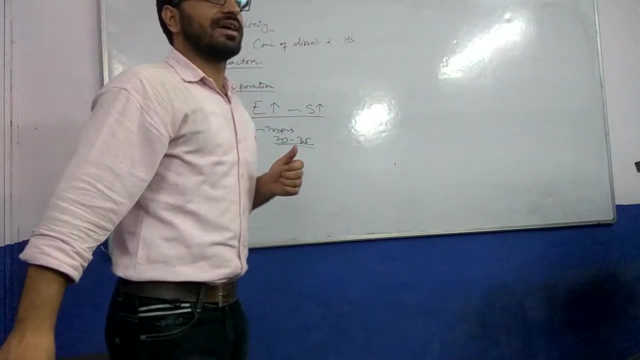 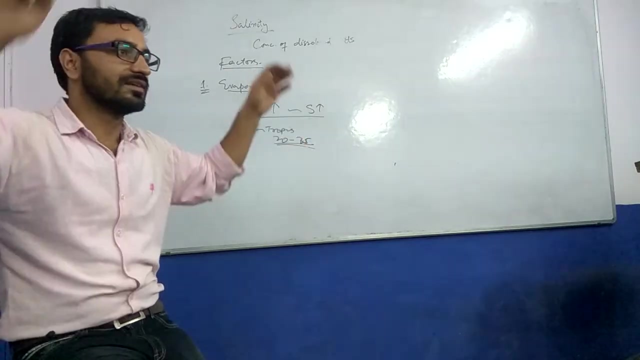 a little below tropics. a little above tropics: 30 to 30 or 35. evaporation is more we have seen in the tropical. in this 30 degrees north and south, there are descending winds. I have studied. descending winds are there. they are dry winds. because of this, evaporation is there, there is more evaporation, there is more evaporation. so if evaporation is more, salinity will be high. therefore, that is the reason why 30 degree has high salinity. that is the reason why 25 or 30. 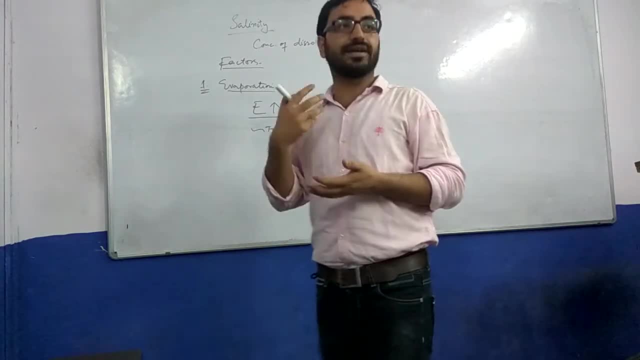 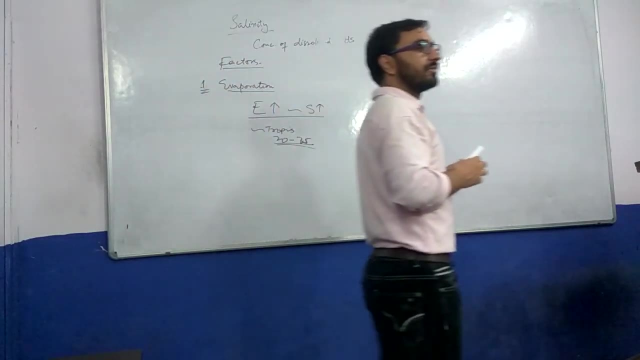 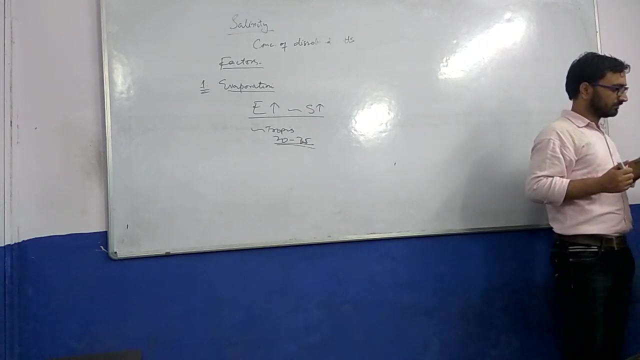 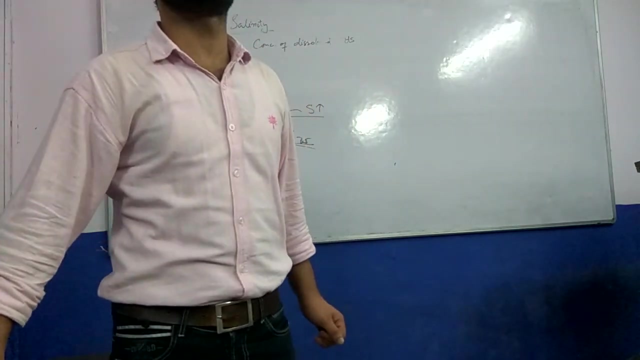 or 35 is the- you know- area where the ocean water has high salinity because there is more evaporation. there is more evaporation. that is the reason for this. that is the reason why equator has low salinity, why equator has low salinity. 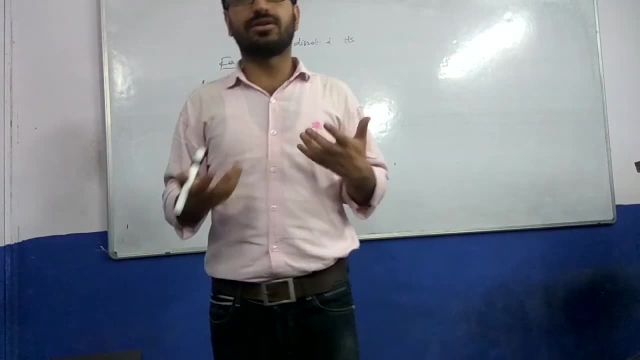 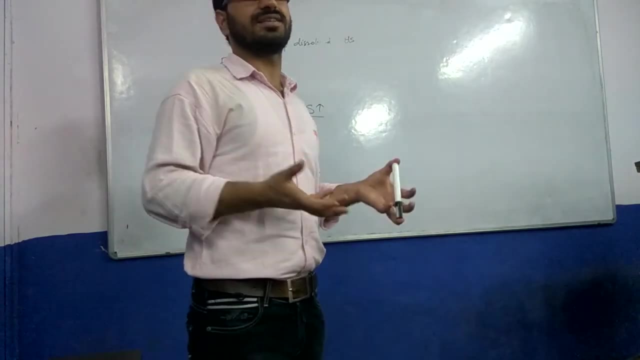 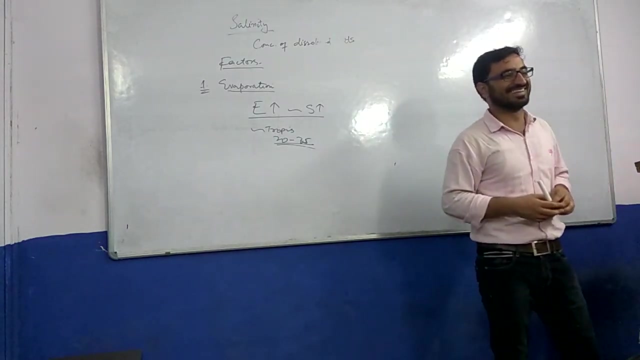 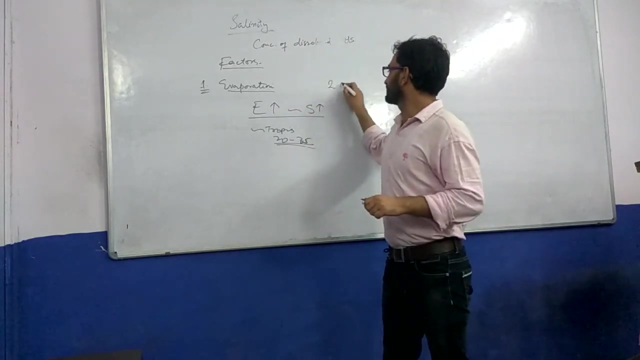 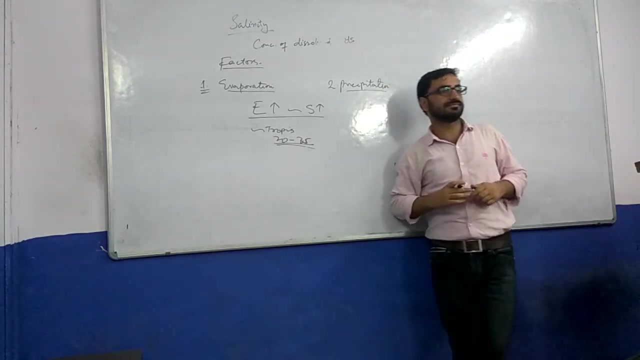 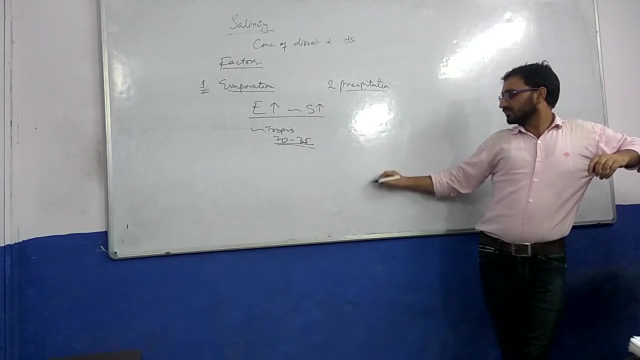 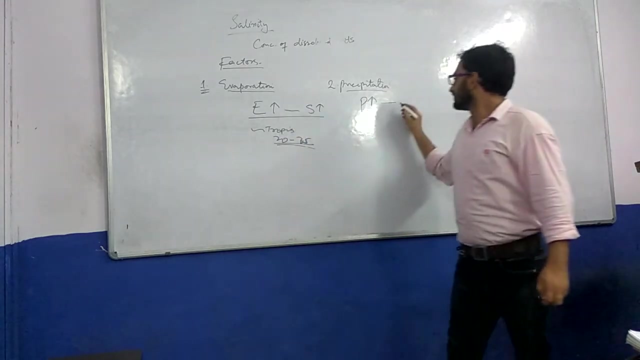 because we have cloudy sky there, we have humid- you know- atmosphere there. because of this there is low salinity. humidity is more here, it is coming. it is coming then after evaporation. second factor is precipitation. what will happen with precipitation, say? if precipitation increases, precipitation, salinity will. decrease. why? addition of fresh water, rain water, precipitation is the pure water, so salinity will decrease. now what you are doing, you are adding water in your vegetable. salinity will decrease, right? so this is the reason i have just told you that equator has low salinity. 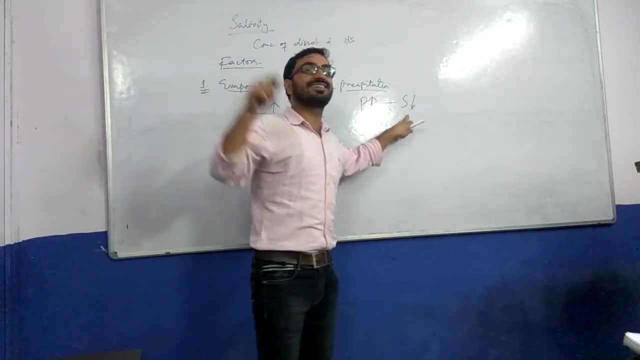 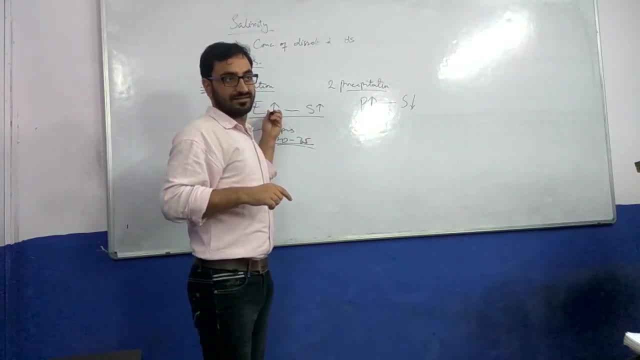 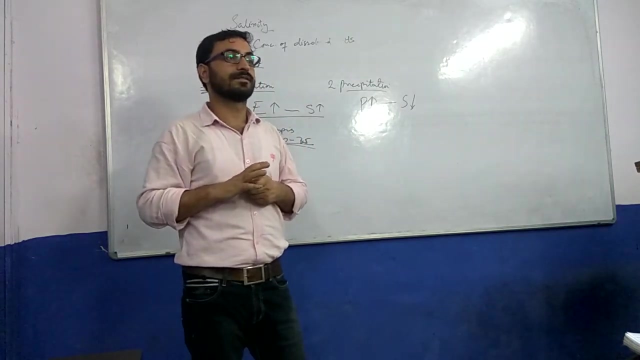 equator has more precipitation. this is the reason why there is less salinity. this is the reason why 50 degree has more salinity, why equator has less salinity. this is the reason. so if we have the areas where the rainfall is high, so in those areas we have salinity. 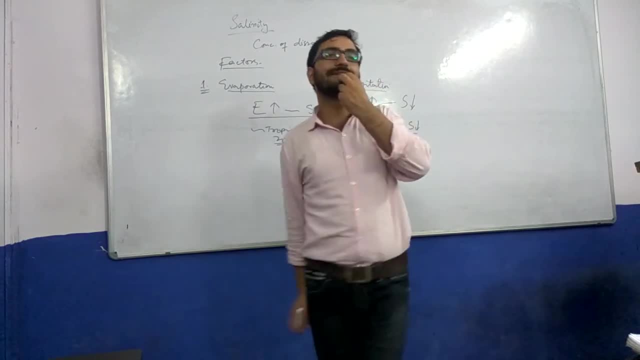 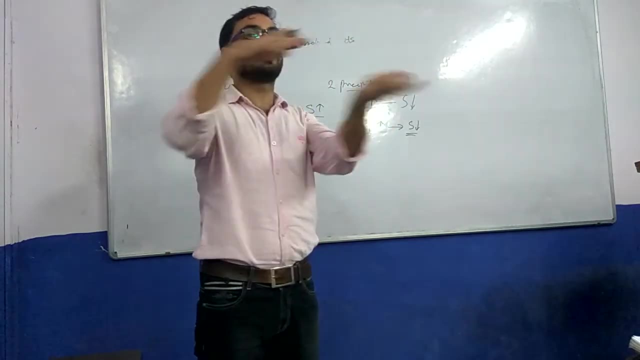 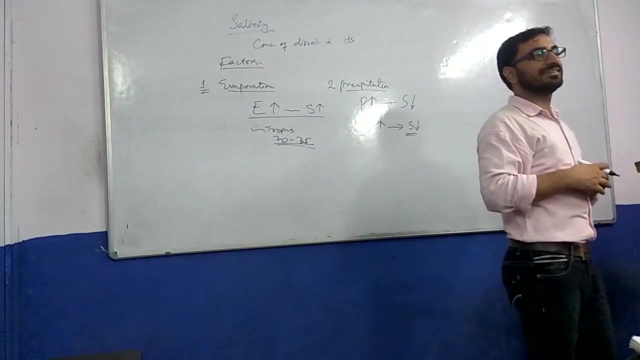 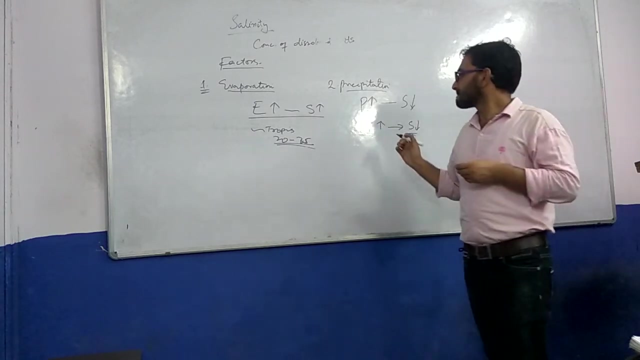 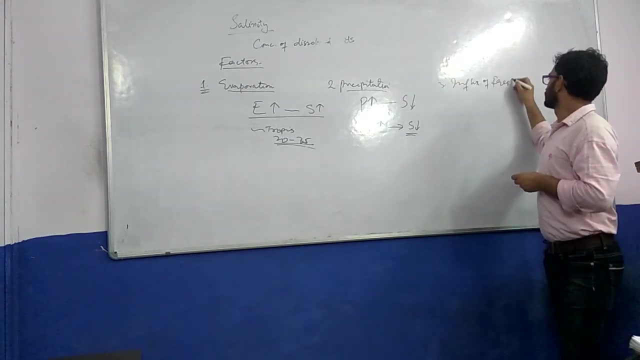 less, less salinity. i have also told you that eastern margin of the ocean and eastern margin of the ocean in eastern rainfall is more, in eastern rainfall is less. salinity will change then. third point here is influx, influx of fresh water. so what will happen with influx of fresh water? 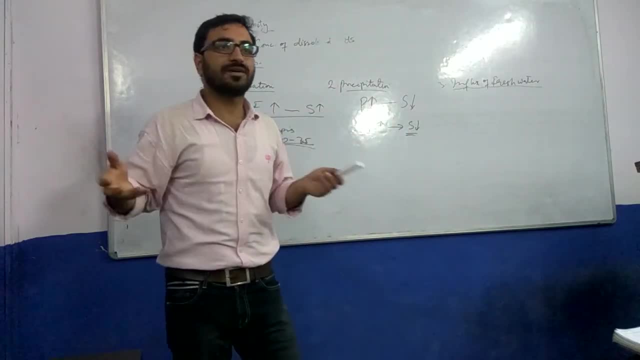 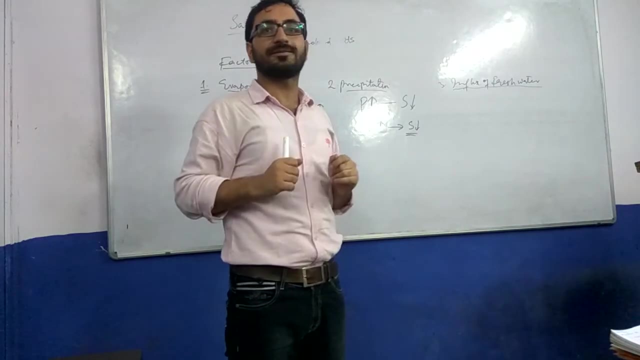 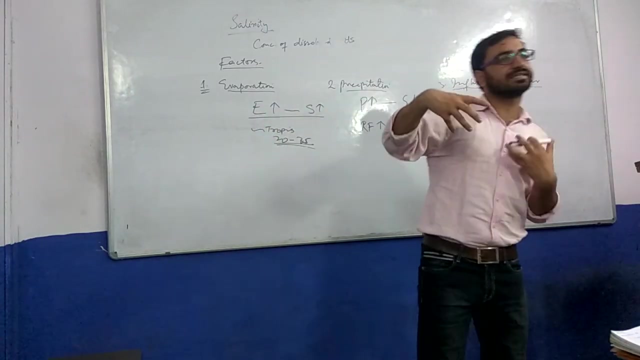 salinity will decrease because fresh water will be added. Ganga river: if you go to the mouth of the river, you can see. salinity will decrease. salinity will decrease. salinity will decrease, you can see if you go to a beach where no river is flowing. 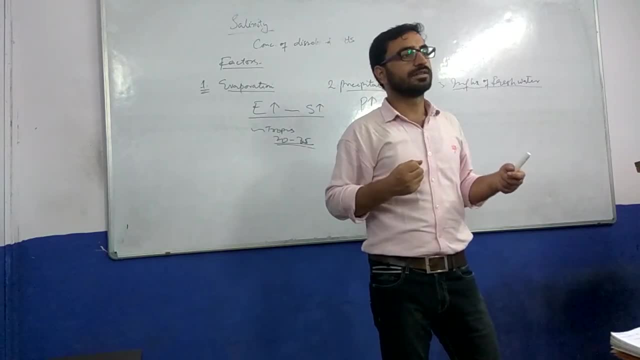 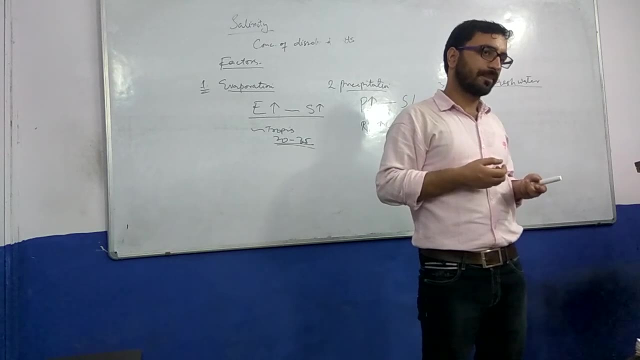 you can't taste that water, then go to some other area where lot of rivers you know influx into the ocean. you can easily taste that water. see the difference between Kondichiri and Chennai. you will feel the difference there. you will feel the difference there. so again, 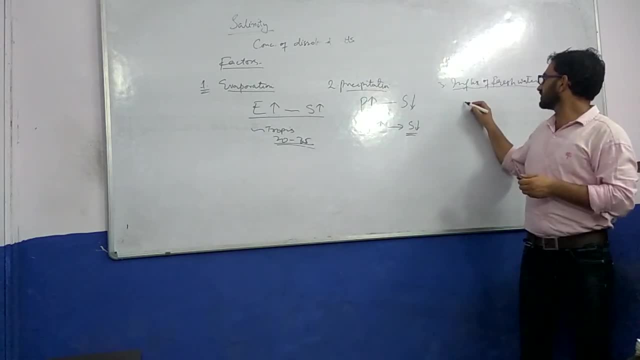 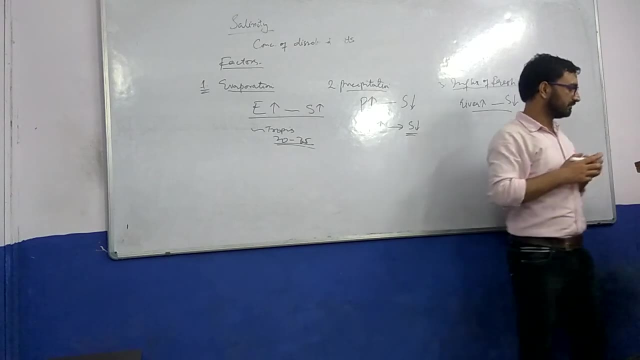 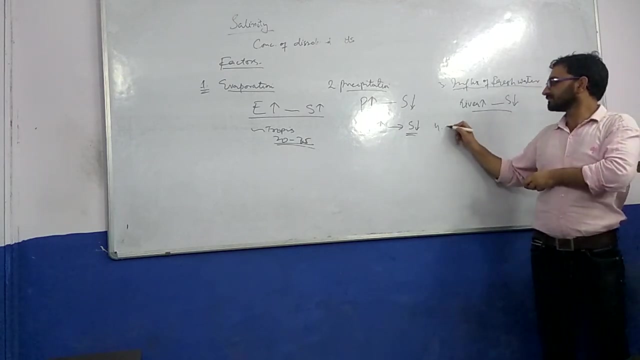 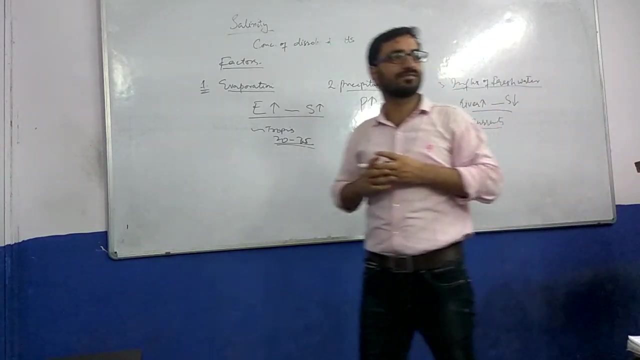 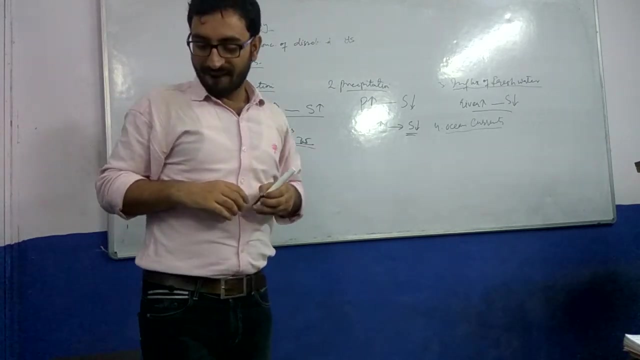 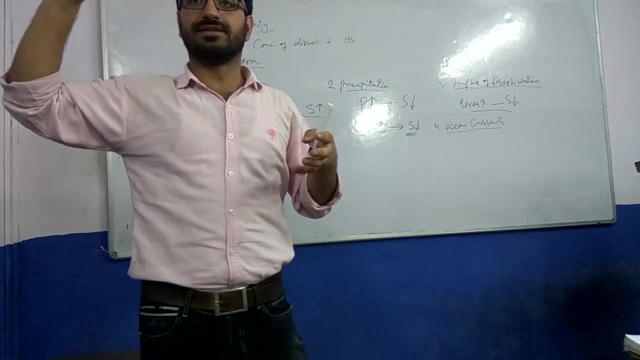 the fresh water is being added, so river water will increase. salinity will decrease. then another factor is the ocean currents. the ocean currents. what will happen with ocean currents? what will happen with ocean currents? what we have seen? that we less salinity in the polar regions. let me tell. 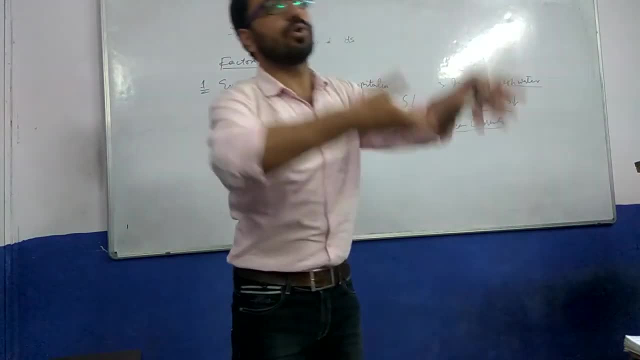 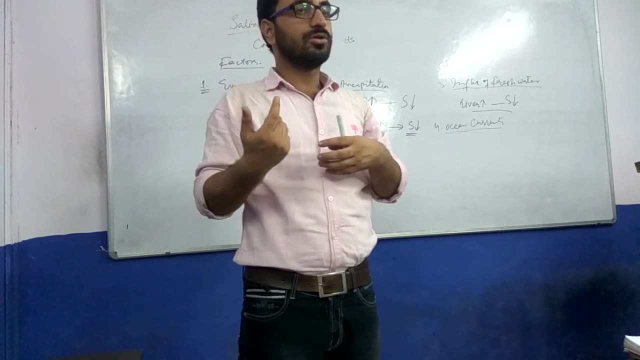 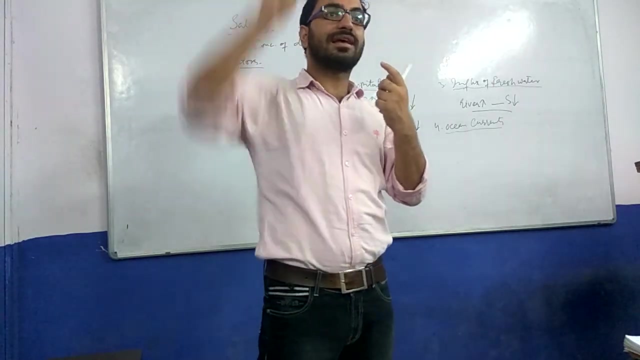 why there is less salinity. so the equatorial water goes there. the tropical high saline water goes to the polar regions in currents, So it increases the salinity there. On the other hand, you see the Labrador current, Labrador current comes, It is the Labrador current. Where does it come from? 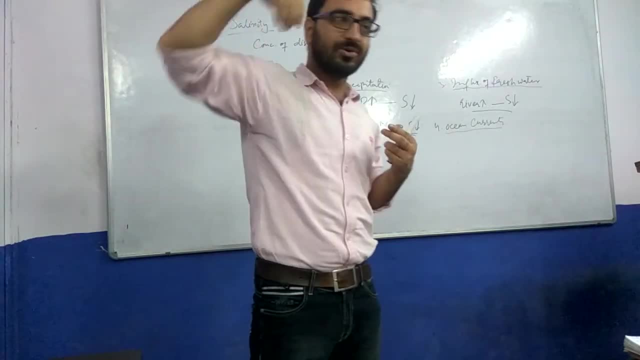 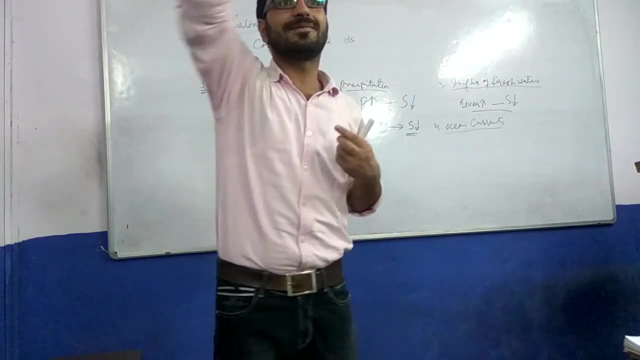 Here, Not the Atlantic mag. It comes from port water circulator. It is the result of the melting of the ocean as well, Melting of the glaciers as well. So this will decrease the salinity. This will decrease the salinity. So there is difference between the salinity in the North-East Atlantic Ocean and North-West Atlantic Ocean. In the North-West, the Labrador current comes and decreases the salinity And in the North-East, the North-Atlantic current goes and increases the salinity. 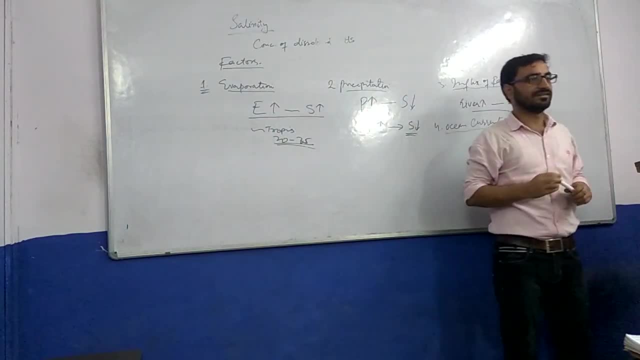 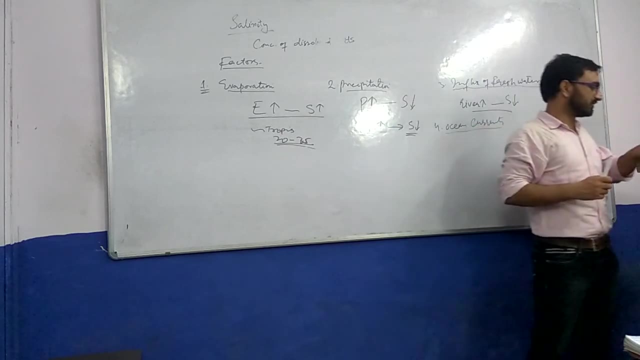 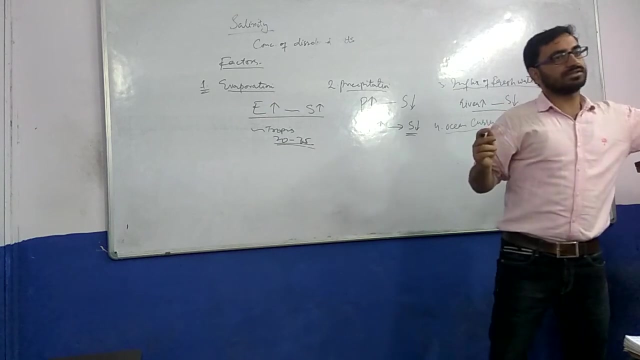 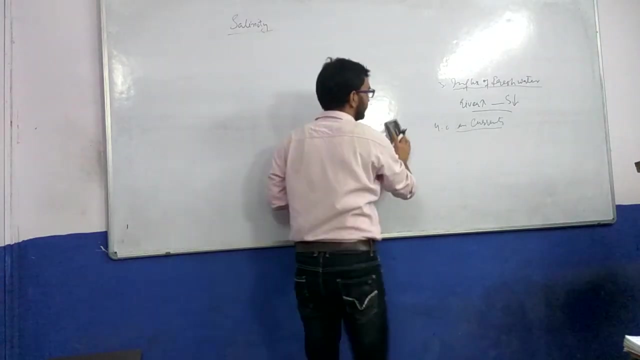 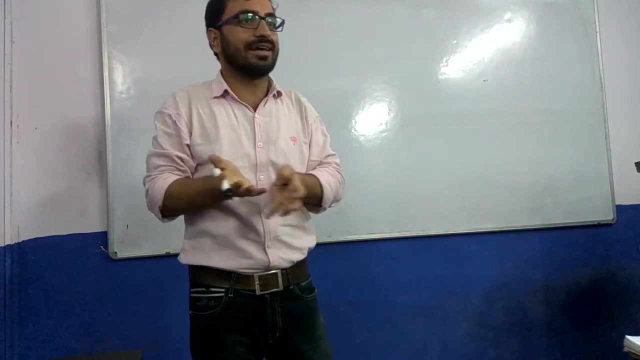 If you have the current in your mind, then you will understand. Otherwise, you will be left behind, You will forget. So if we see the horizontal distribution of salinity, One more point to remember: The marginal ocean, the marginal sea. will its salinity increase or decrease? 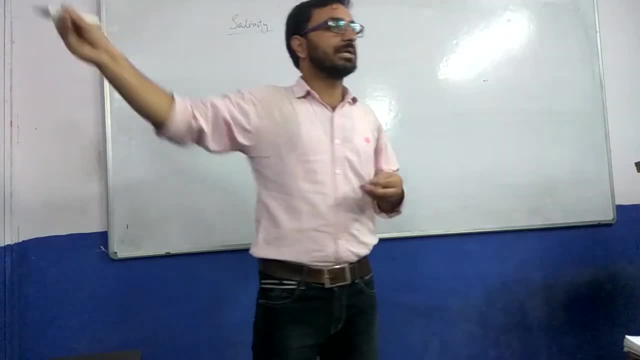 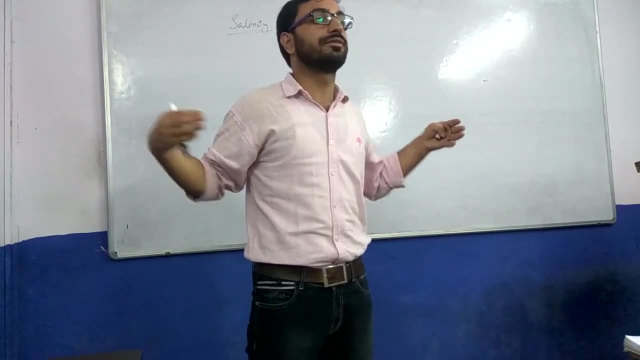 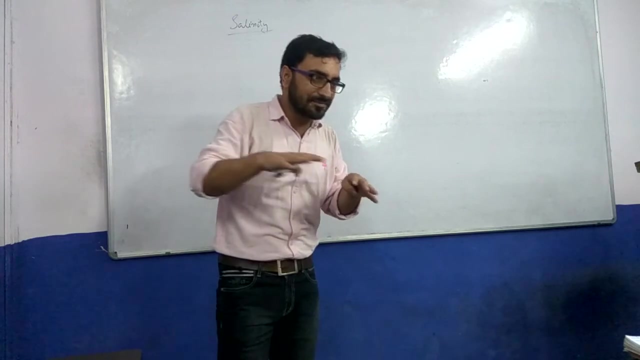 It will decrease Because addition of fresh water through rivers: It is the addition of the fresh water. The addition of the fresh water through rivers decreases as you go away from the margin. It is impact decreases. Fresh water is created at the margin. 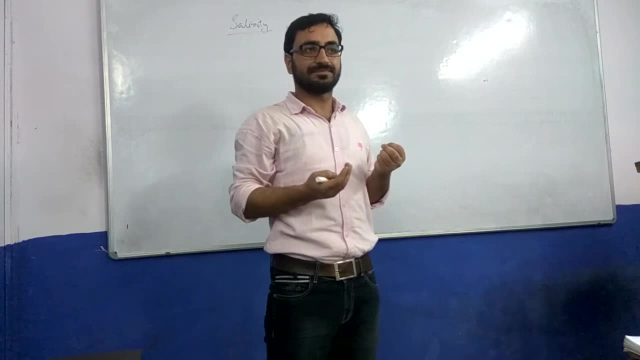 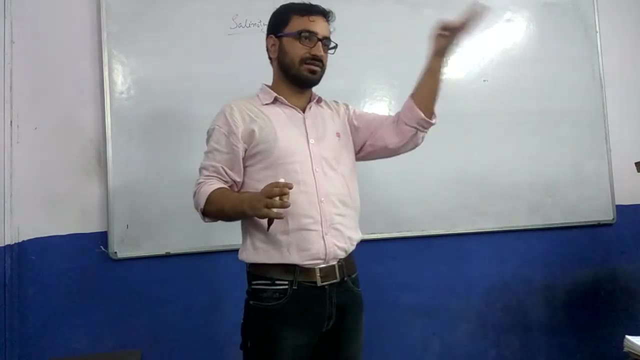 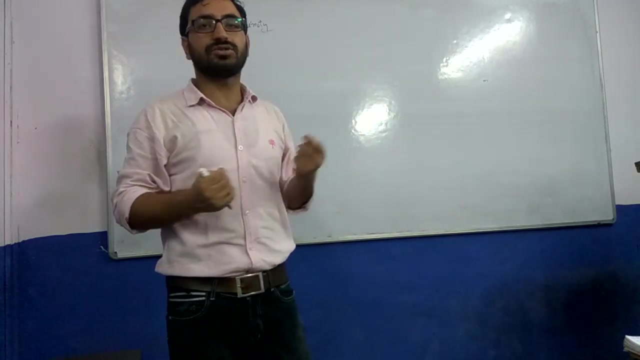 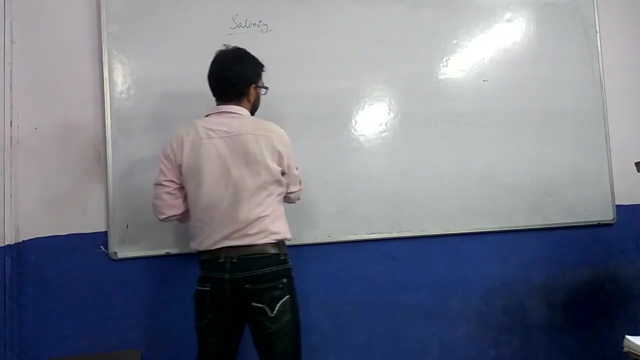 Once you go inside the ocean, the effect of this fresh water will decrease, So marginal area will be having low salinity As compared to the center of the ocean. You can make this point yourself Now. you are mature in oceanography. Now let there be some graphical representation. 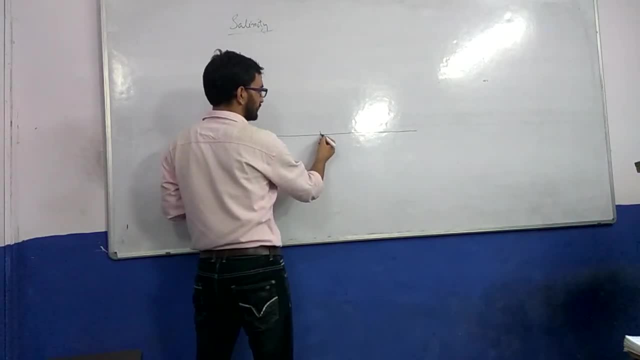 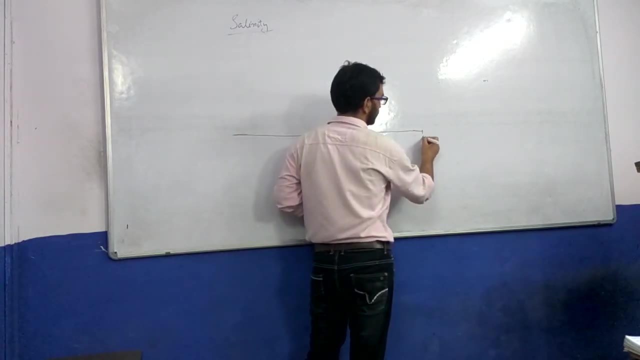 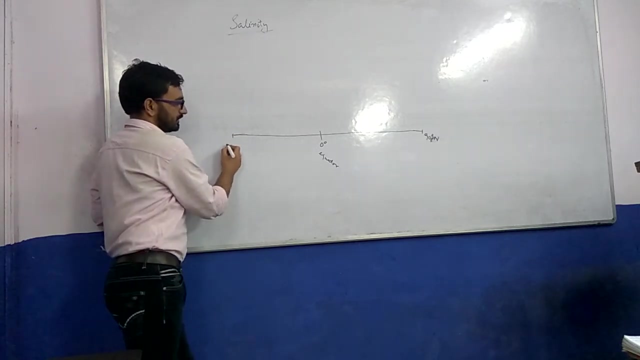 Let me take the case of the equator here, Zero degree, And let this be the north pole, Or 90 degree north And this be the 90 degree south. This is southern hemisphere, This is northern hemisphere, And accordingly we have 10,, 20,, 30,, 40,, 50,, 60,, 70,, 80. 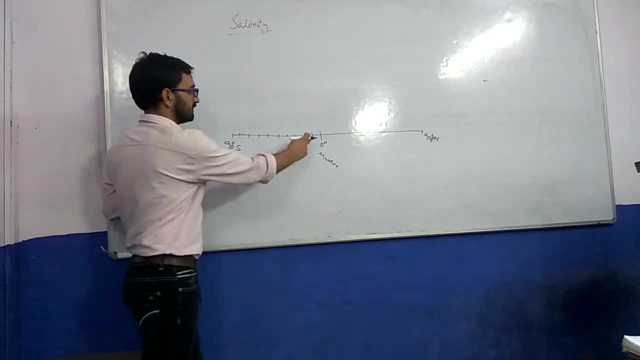 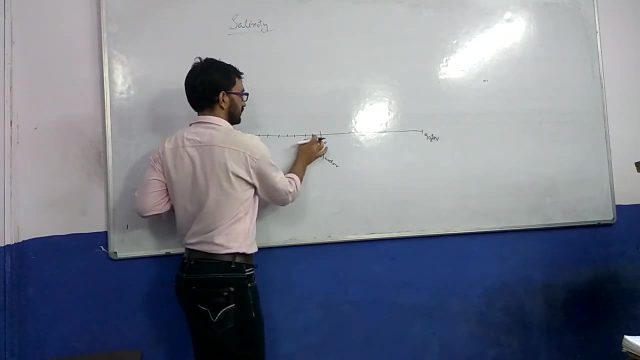 So 90 degree. Ok, Another wave. So this is northern hemisphere. Like this: 1, 2,, 3,, 4,, 5,, 6,, 7,, 8 and 9.. So like this, One dvd and dvd is dvd and dvd is dvd. 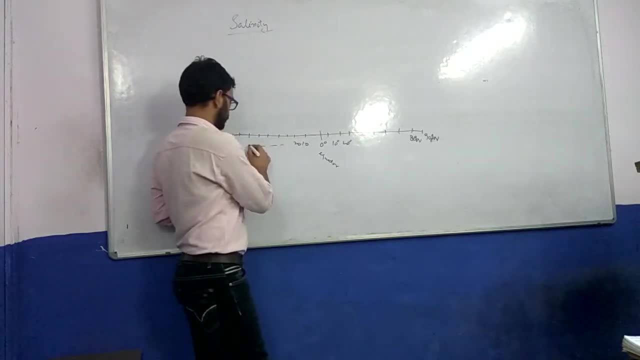 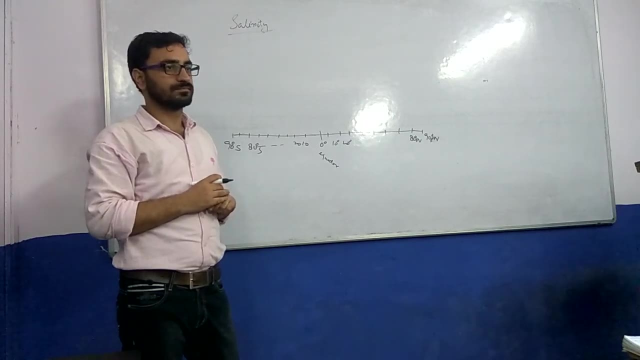 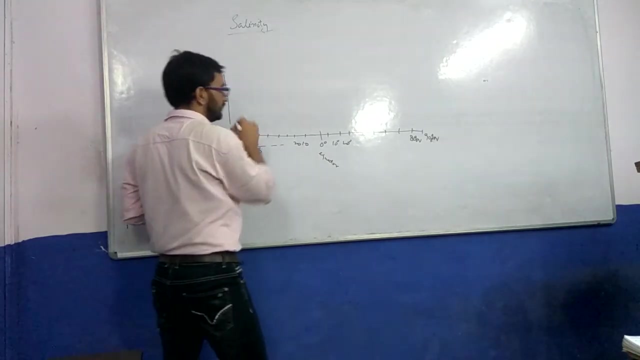 One dvd and dvd is dvd. One dvd and dvd is dvd Two, Three, Four, Five, Six, Seven, Eight, Nine, Ten, 11., 12., 13., 14., 15., 16. 17.. 18., 19., 20., 21., 22., 23., 24., 25., 26., 27., 28., 29., 30., 31., 32., 33., 34.. 35., 36., 37., 38., 39., 40., 41., 42., 43., 44., 45., 46., 46., 47., 48., 49., 49.. 50., 51., 52., 53., 53., 54., 55., 56., 56., 57., 58., 58., 59., 60., 61., 62., 63.. 62., 63., 64., 65., 66., 67., 67., 68., 68., 69., 69., 70., 71., 72., 72., 73., 73.. 74., 75., 76., 76., 77., 78., 79., 78., 79., 80., 81., 82., 83., 82., 83., 84., 84.. 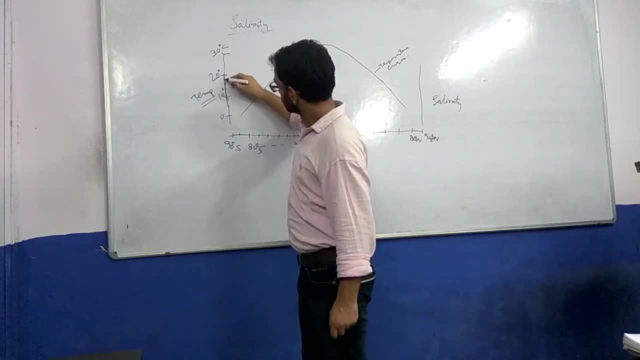 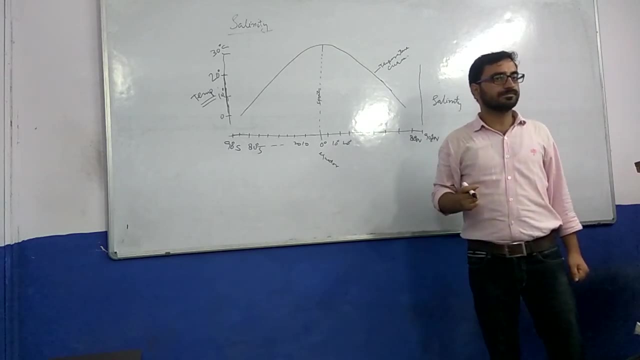 85., 86., 87., 86., 87., 88., 88., 89., 90., 90., 91., 92., 92., 93., 93., 94., 94.. 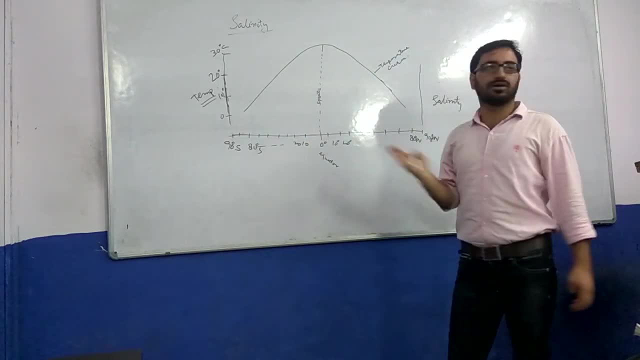 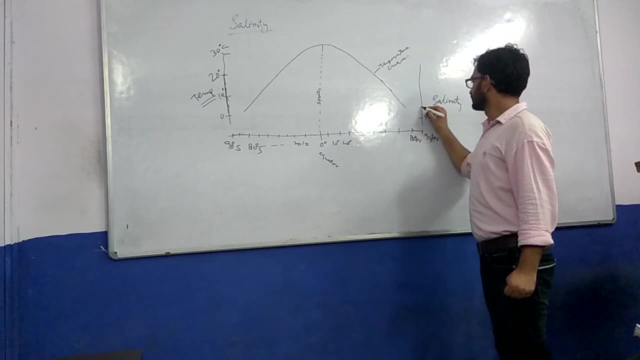 95., 96., 96., 97., 98., 99., 100., 100., 100., 100., 95., 100. 11. 120., 120., 129., 12.. 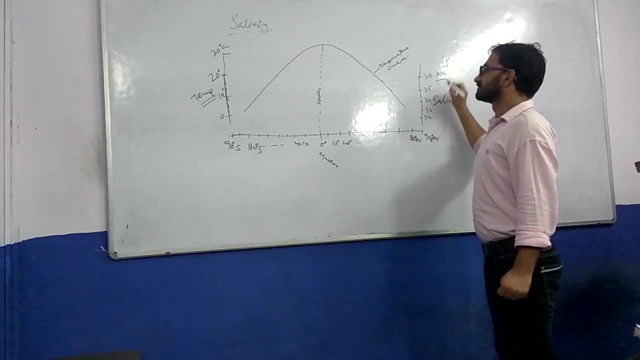 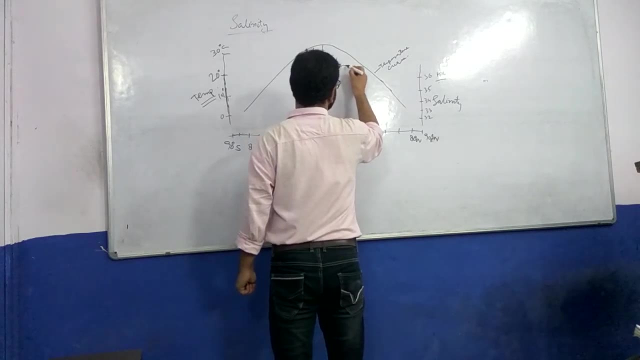 120.. 149.. 14., 120.. 14., 14., 14., 15., 15., 16., 16., 17., 18., 19., 19., 20., 21.. 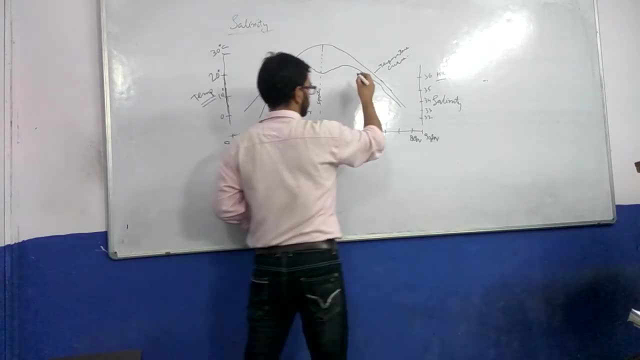 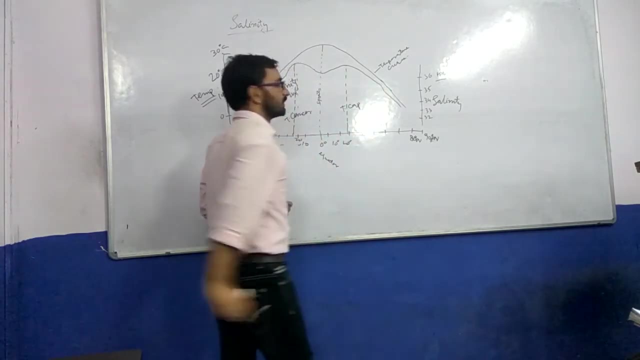 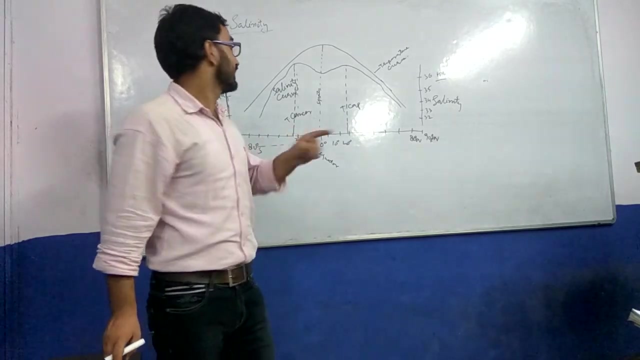 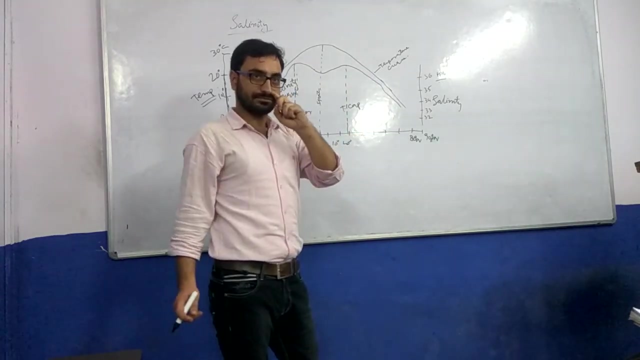 22., 23. 24.. When the salinity is maximum- 25,, 28,, 30,- we will not solve it. salinity maximum at: we are at about 36, when it decreases towards this, it decreases towards this may samajh. 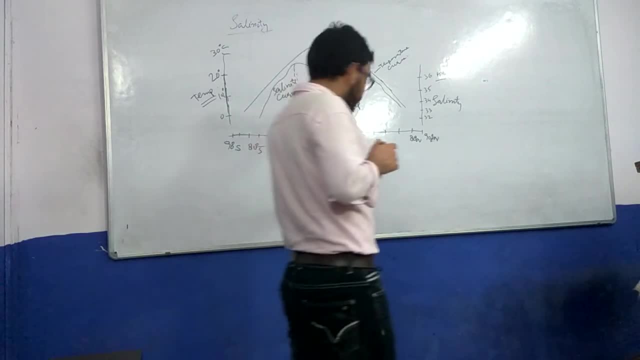 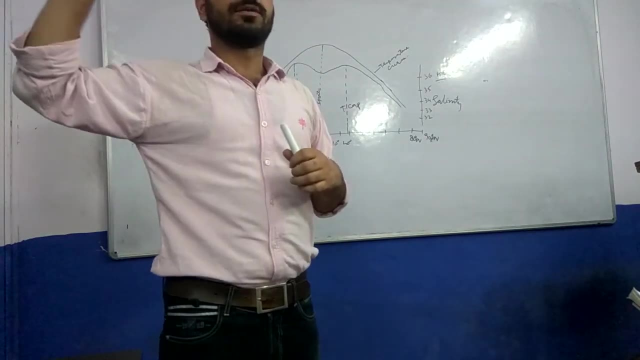 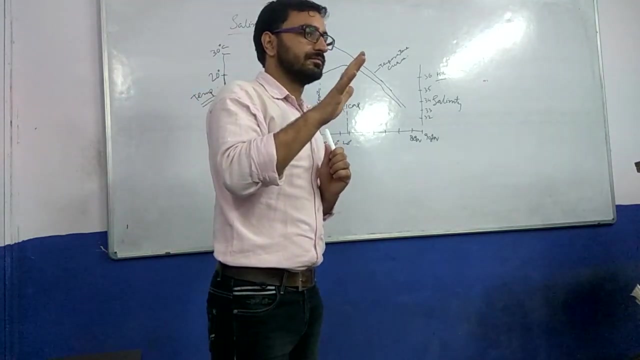 rahe ho, na samajh rahe ho. so this point ko hum kaise dimaag me pithayenge? the salinity of the ocean water decreases when we move from equator to the pole. samajh rahe ho? 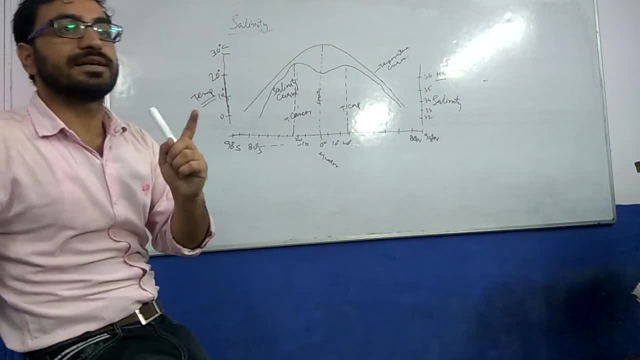 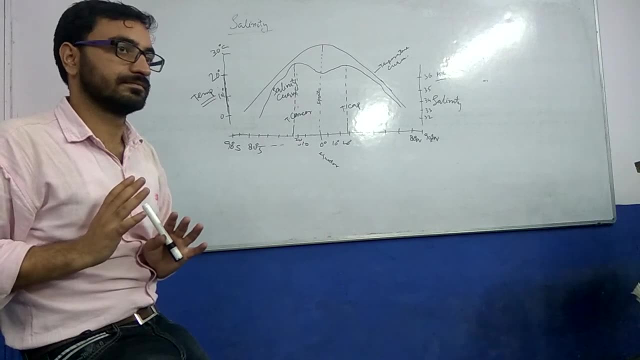 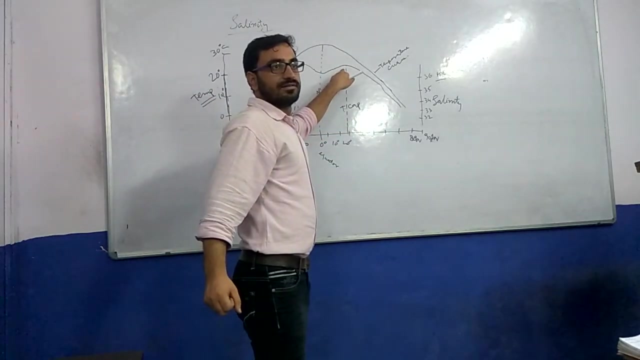 general statement: sarvesh general statement is that salinity decreases when we move from equator to the pole, Or it increases when we move from pole to the equator, And there is the exception. there is exception: maximum salinity is not equator. It is tropical. see the statement is this: salinity decreases from equator to the pole. this is correct statement. this is true statement. Salinity decreases from equator to the pole. this is correct statement, but from. if this statement is correct, 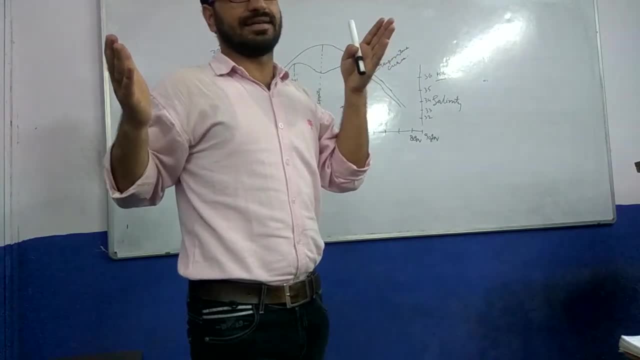 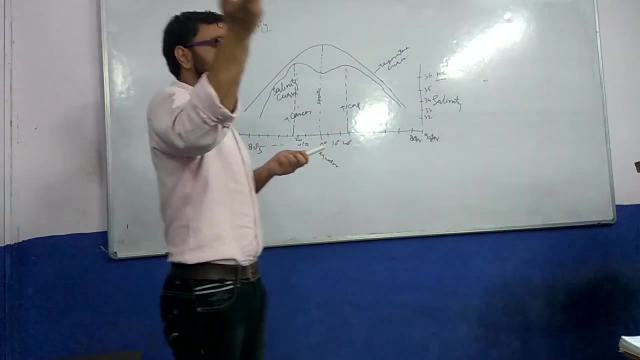 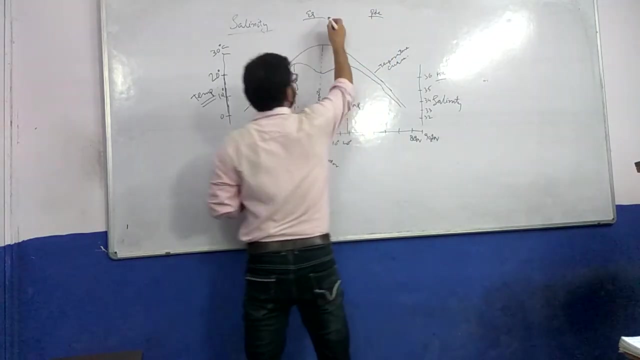 then maximum salinity should be at the equator. but it is not like that. the maximum salinity is at 30 degree. both statements are same. so if I make a rough data, let me make a rough data over here. here I am taking equator and here I am taking pole. 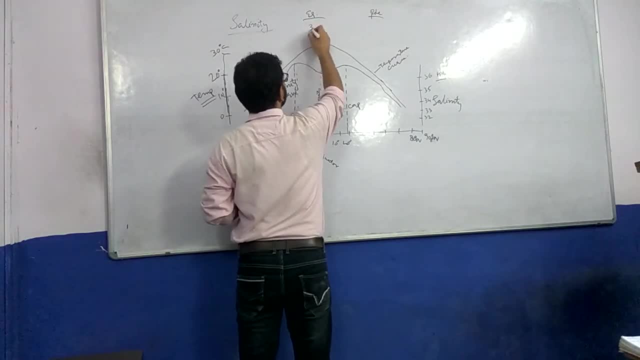 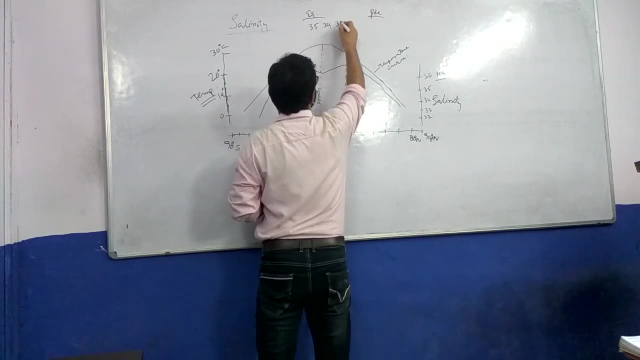 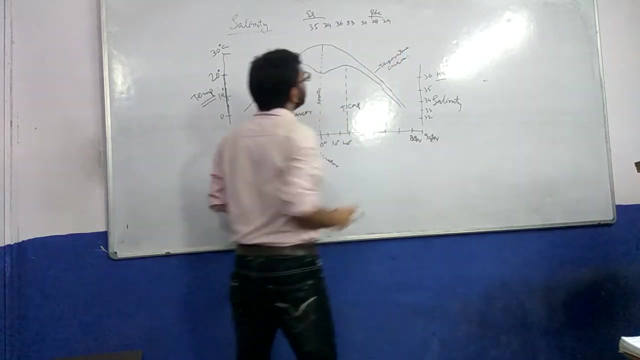 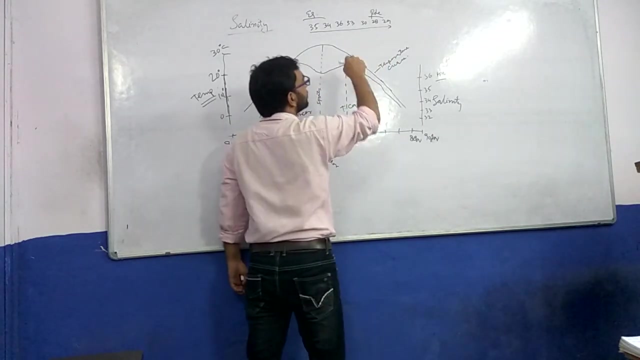 I will give you the rough data. the salinity is like 35,, 30,, 4,, 36,, 33,, 30,, 28,, 29. let it be like this now. you see, there is a trend that it decreases from 35 to 29, but there is the 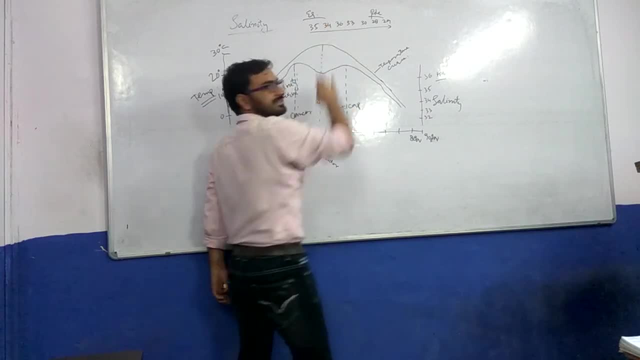 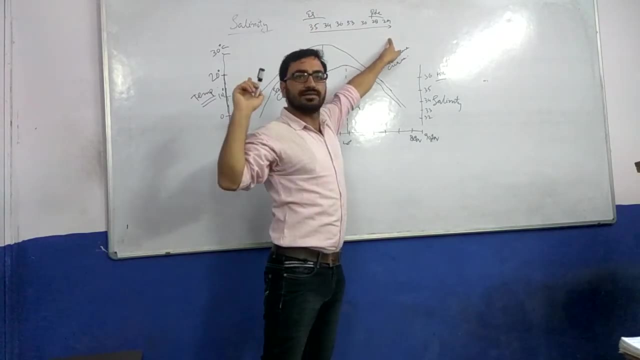 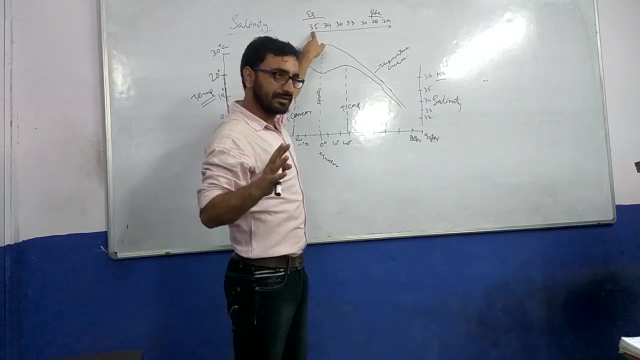 exception, one exception where it increases. so my general statement is true that it decreases from equator to pole. this is correct. but this statement has one limitation: that it does not mean that maximum is at equator, it is at properties. that is why I have shown this like this: 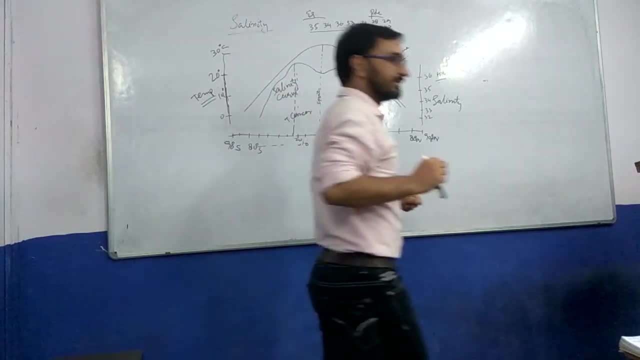 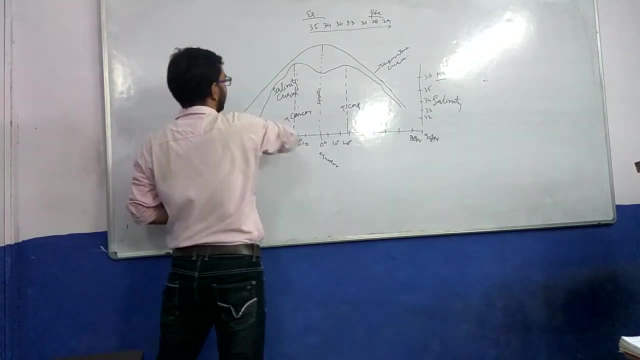 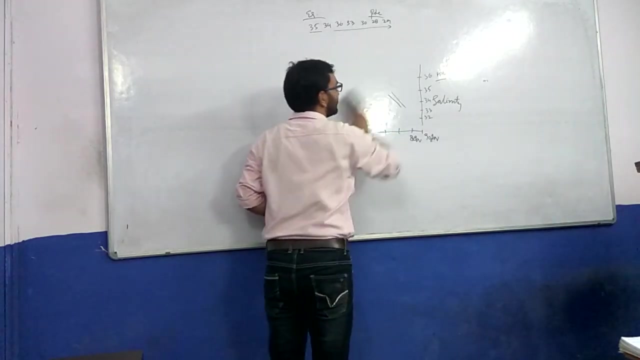 this is the horizontal distribution. are you sleeping? if you want to sleep, tell me, I will make you sleep. who wants to sleep? I will make you sleep. ok, ok, it is done. ok, I do not need to sleep for one more second. I will sleep with somebody else. 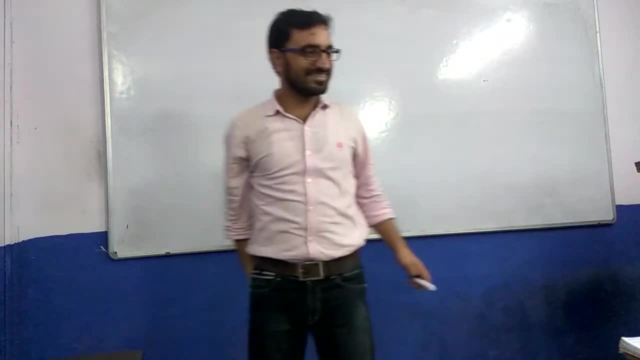 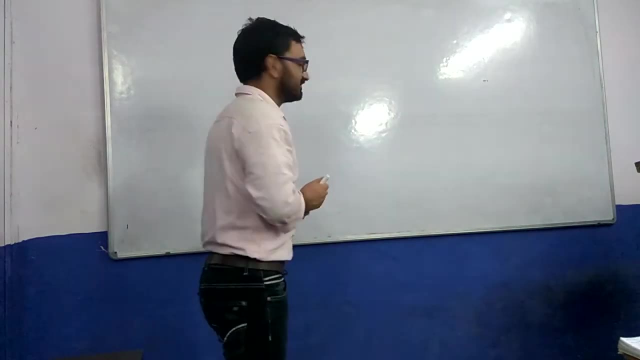 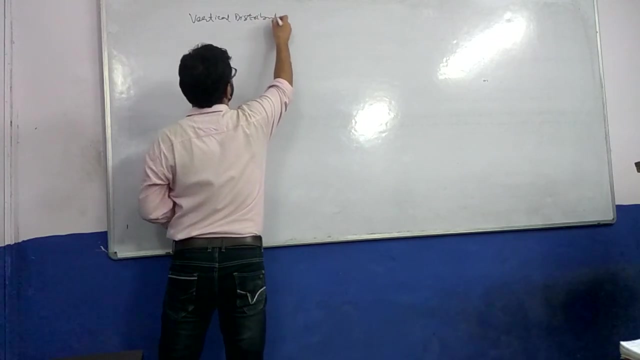 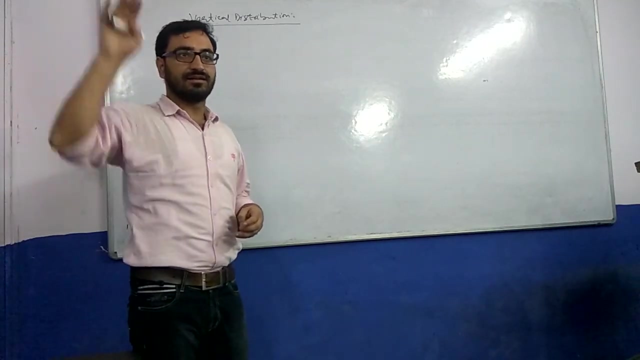 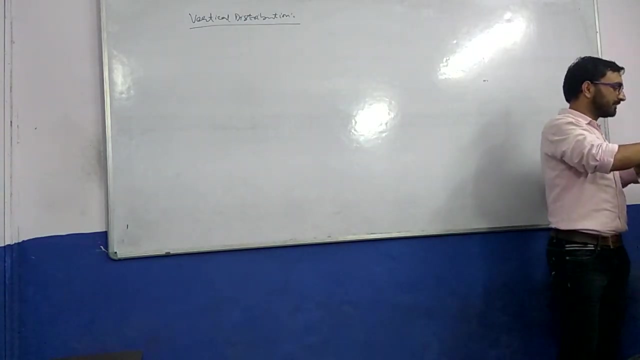 sleep with me, sir. did you tell it is 34.5? this is average. hmm, average. ok, let us see multiple distribution. ok, I have given two diagrams of temperature and density. do you remember that? Do you have it in your mind? Let us draw the vertical distribution of salinity. 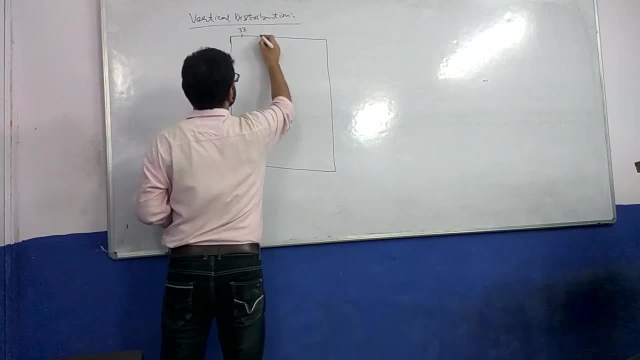 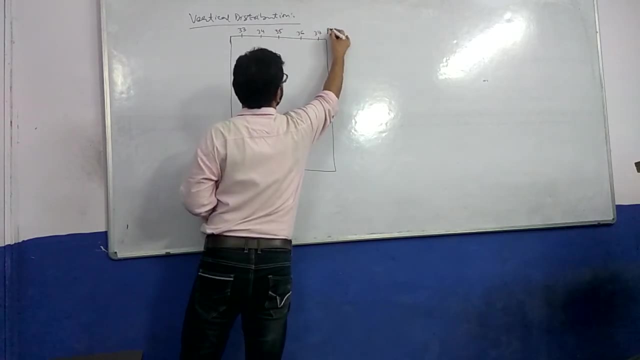 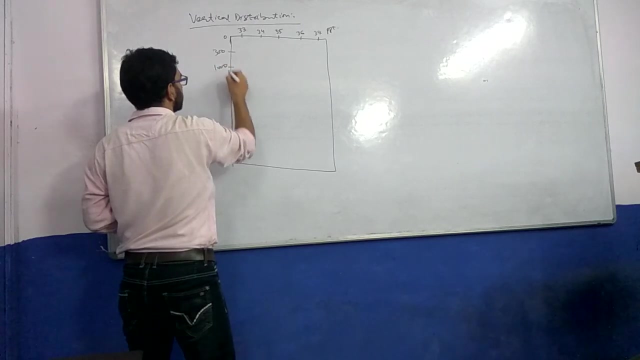 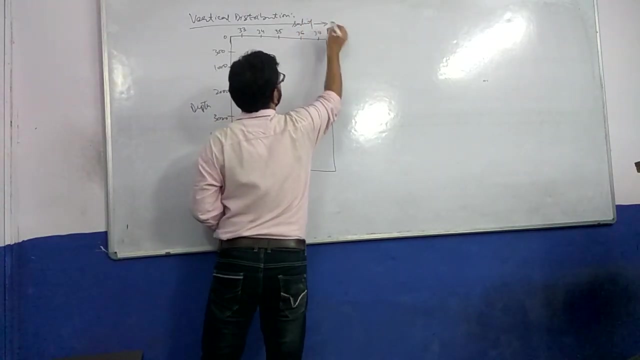 This is circle. this is 300, this is 1000, this is 1000, this is 1000, this is 100.. This is salinity, Salinity, This is the salinity. Salinity is this way. 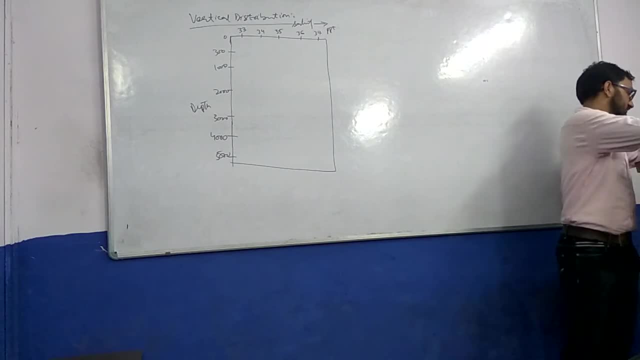 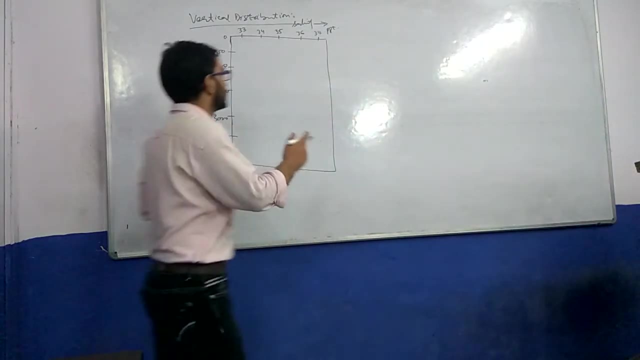 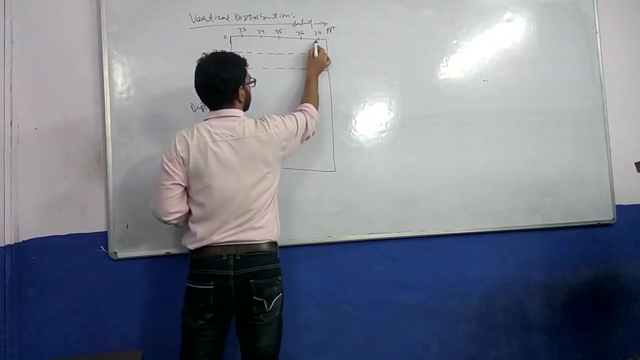 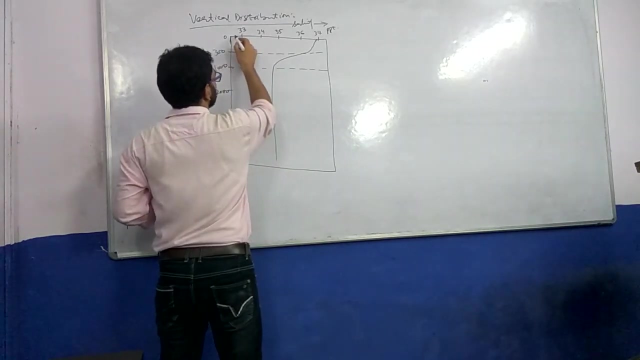 I will cover. So I will draw this fast and we will then discuss it. So exactly the same is the case here, But here what happens is that salinity decreases, then abrupt decrease, and goes like this: Salinity In case of air they never have to increase- and then it goes like this: 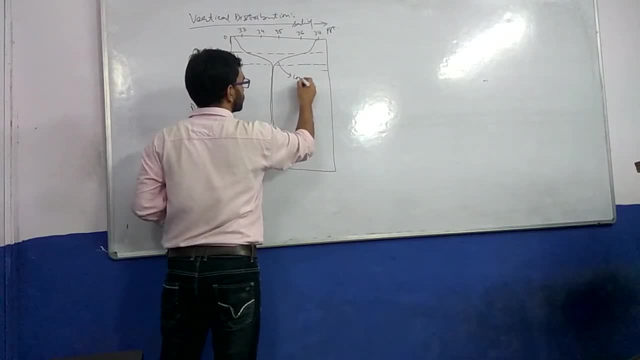 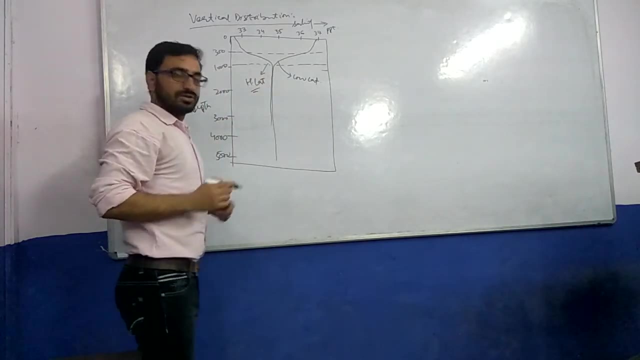 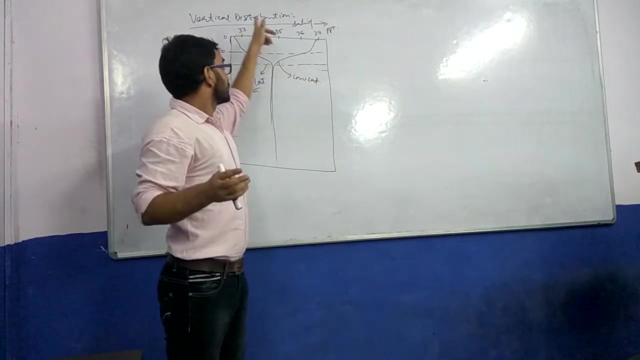 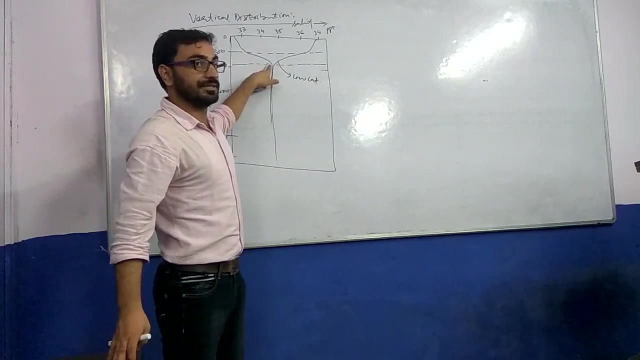 This is more latitude, so this is higher latitude. So here, in the case of temperature and in case of the density, the higher latitude area was not showing any change. But in case of salinity, there is increase in the salinity in the higher latitude. There is decrease in the salinity in the lower latitude. So I have the surface area where there is high salinity in the lower latitude and low salinity in the higher latitude. Try to understand the concept. This is the surface water. There is high salinity. 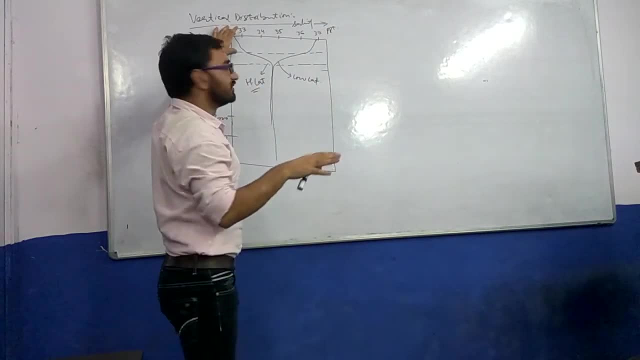 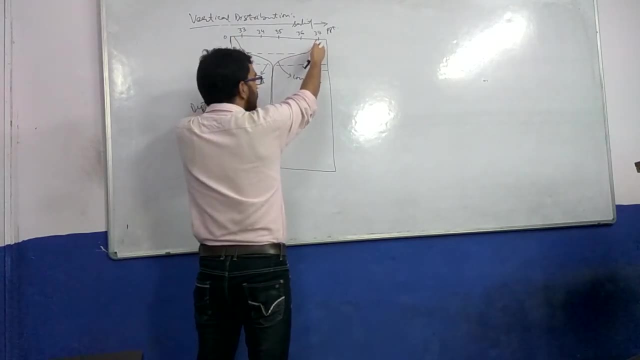 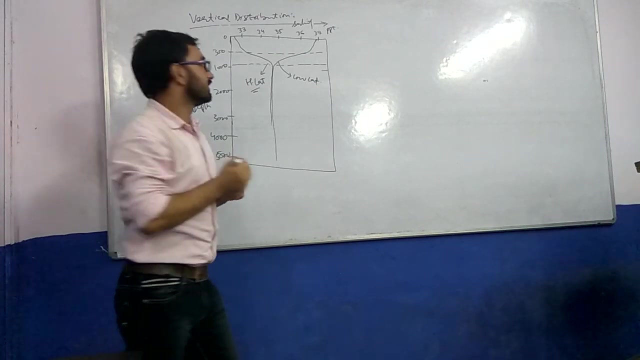 Salinity in the higher latitude and there is more salinity in the higher latitude, Then the salinity starts decreasing or increasing here. Then there is abrupt decrease, there is abrupt increase and then it remains constant. This is called hallowed line. Line means sharp change. 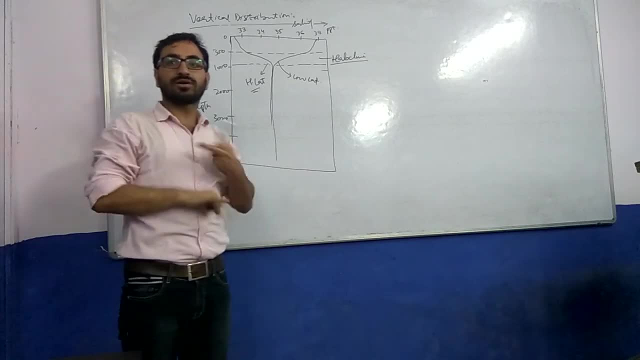 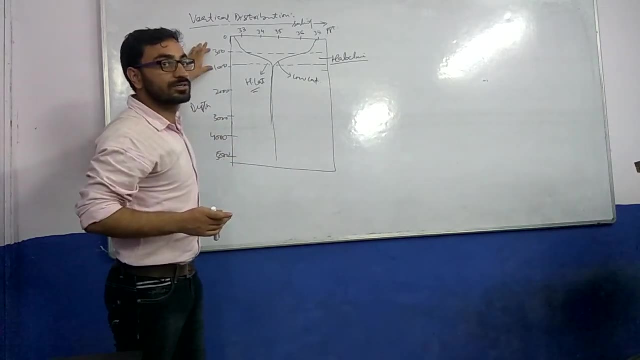 Hallowed means sharp, Thermocline, hypnocline, halocline. All the three represent 300 m to 1000 m depth in the water column. All the three represent this depth, 300 m to 1000 m. But thermocline: sharp change in the temperature, fall in the temperature Density, rapid increase in the density, hypnocline: Here halocline is increased, sorry, decrease, hydrolyzed increased. If you go to the extreme southern Atlantic Ocean, what you will see is the top water and the bottom water just 200-300 meters below. the salinity will increase. I am talking about the Atlantic Ocean. you go to the extreme south of the Atlantic Ocean. the salinity in the surface. if you go down, the salinity will increase. If you come to the equatorial area of the Atlantic Ocean, come to 20 degrees, come to 15 degrees, the salinity at the top and bottom will be different and it will decrease.